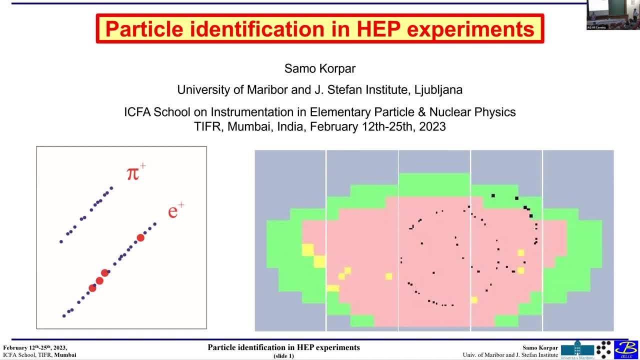 Scintillator detector, solid-state detectors and this position-sensitive particle detector, And also he worked for the multiple proportional chamber, So he has a wider view of all the detectors And to identify the particles you need all the ingredients of all the detectors. 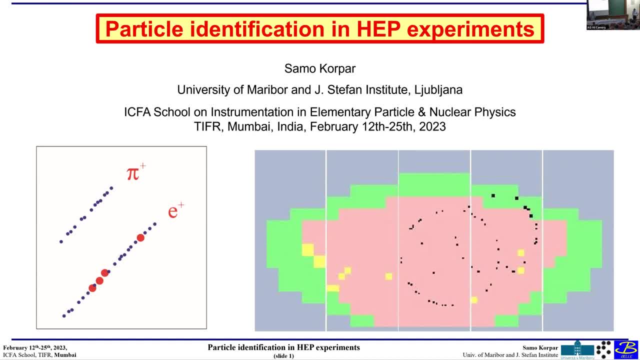 So that's why that he is an expert in particle ID And he is also a co-author of this particle, a book called the Particular Identification Methods. So you can assume that why we choose him to talk with the Particular Identification. And another thing I have to just tell that I told you that the school date is chosen as 12th February because this school was earlier school was holding here in 1993, 12th February. 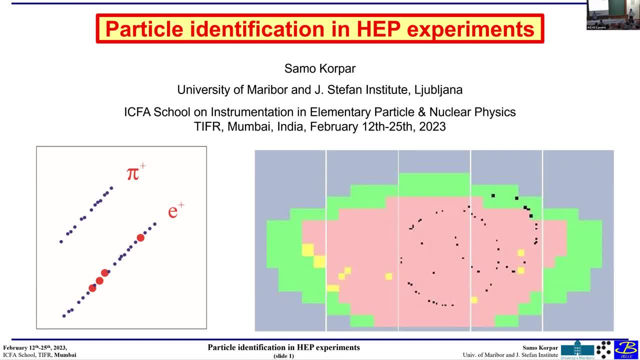 I was one of the participants and he was also another participant in that school. So now that time you are the student, now the teacher. So I hope after a few years some of you will also give a lecture in the first school. 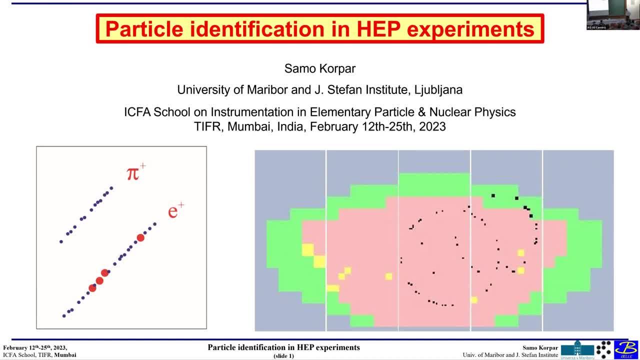 Okay, Samu, Okay, thank you. Thank you very much for this kind introduction. As said, I'm working mainly on the detector development and the mostly rich detectors and all correlated things in the medical science or something else, So wherever we can use our knowledge. 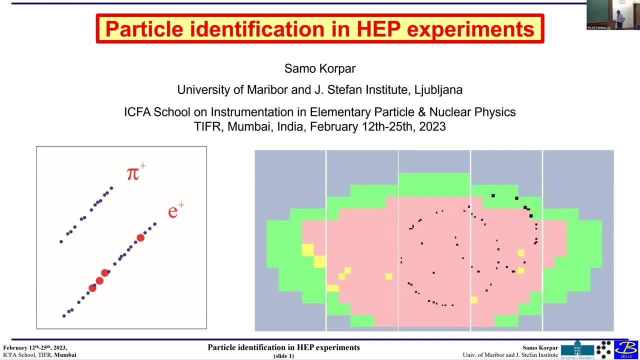 Besides the high energy physics. So today I will talk about the particle identification And here are just two examples basically. So what we do in high energy particle physics: you all know that basically we collide particles and then they decay, most of them very quickly. 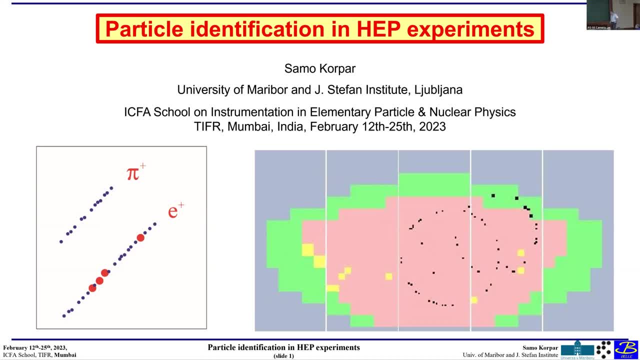 And at the end only a few remains that leave the trace in the detectors And those then leave the tracks In some detectors, then some special high energy depositions that help identify them. Let's say, like in this case, or we have a specialized detectors that actually serve more or less only the purpose of identifying or discriminating between particles. 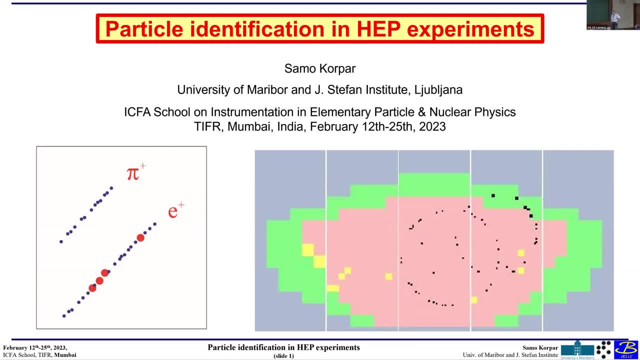 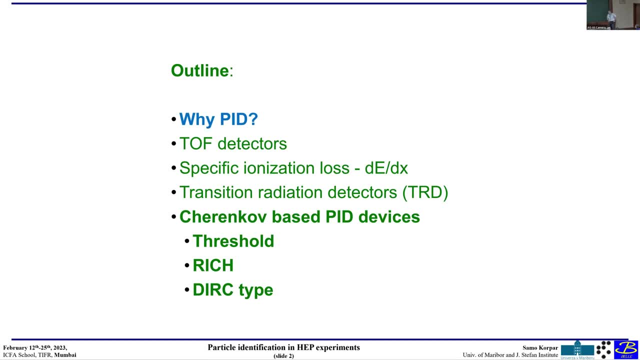 And these are mainly based on the Cherenkov radiation. So we will talk First, we will briefly look at a few Reconstructions where particle ID actually greatly improves the visibility of the final resonance of peak, And then we will go. we will say a few words about on general, about the particle identification. 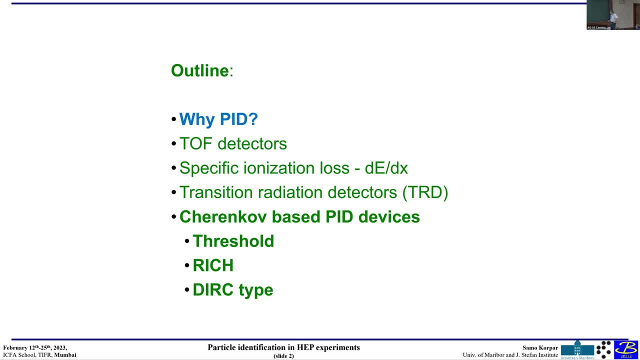 And then we will go to the Through a different type of detector. The first part is actually time of flight. detector is very, very basic concept And it is with us a long time, But as of course has Limitations. And then there are some that are actually also used for other purposes. 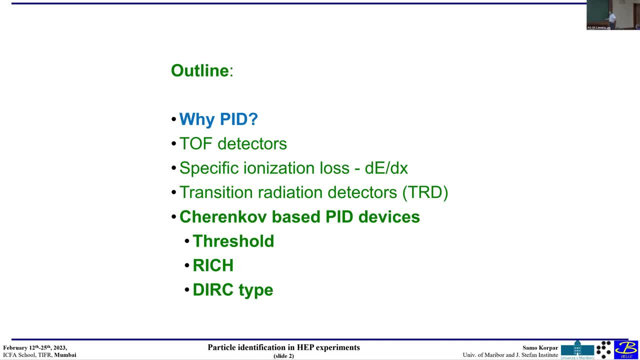 Not dedicated to particle ID And, as I said, the Cherenkov based particle ID devices Are usually Only Installed for the purpose or separating between particles. So, Cherenkov based there is a basic one, threshold one. Then there are imaging detectors and the detectors that 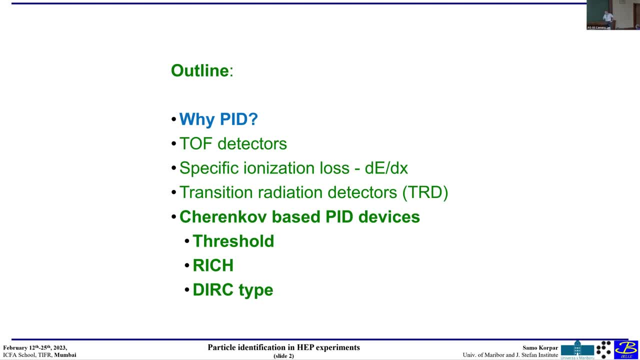 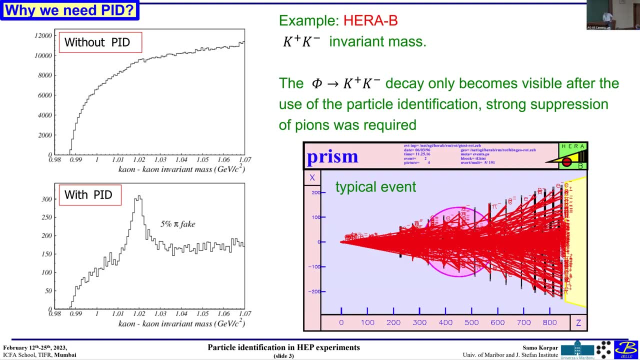 Internally propagates the light Within the sort of a light guy Quartz bar, To the outside of the detector Where there is more space to put Your detection devices. So why do we need? There are a few examples. This is from an old experiment where I- where I started more or less. 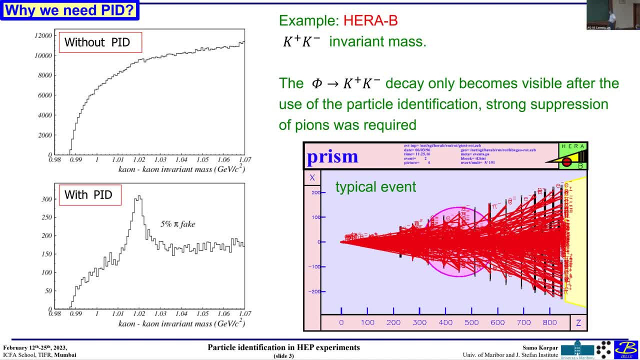 My rich building career, Hera B At the easy. long time ago There was a- We will see Some more slides later At the reach detectors about this Experiment And This was a typical event. Basically, a lot. This was fixed. 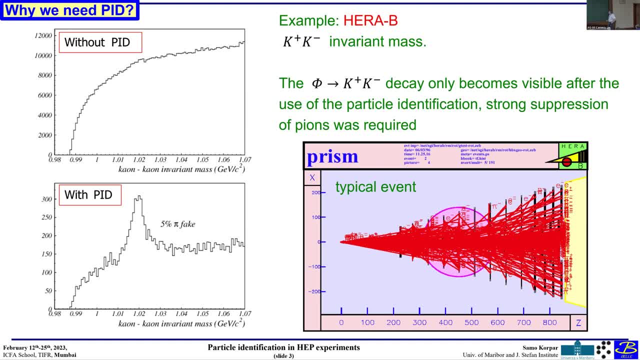 Target Target experiment, Where protons were hitting the wire Inside the beam pipe And then a lot of particles were produced, Many pions In there, And if you wanted to see Okay On, then you really need to have a good suppression. 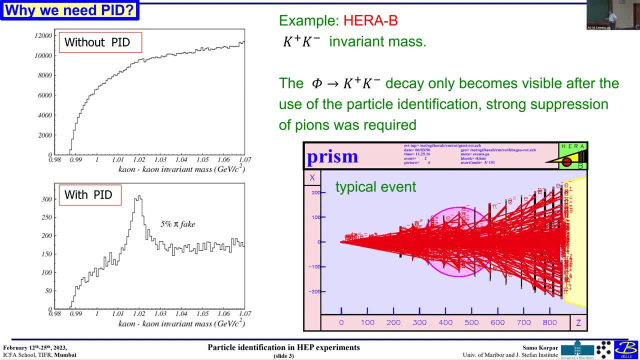 In particular edification. So this was of course. you start with tracks, You pair two tracks together, You calculate invariant mass And You try to see the peak Of the five meson Which is produced from two counts. And if you combine all, including all the pions in the event, you don't see. basically, 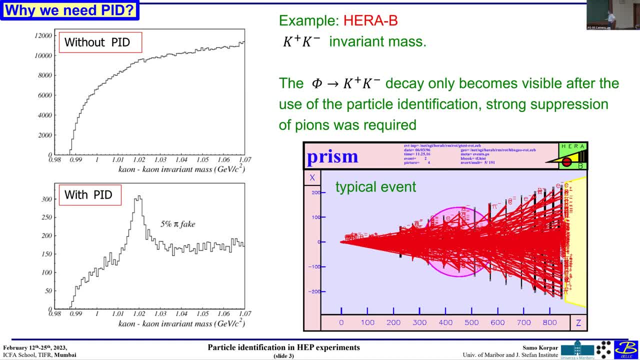 nothing here. But after you apply The selection criteria based on the Charing code detector, You can see that Five peak nicely Sticks out. So this is the Idea. Why do we use it? This is the LACB experiment, where they 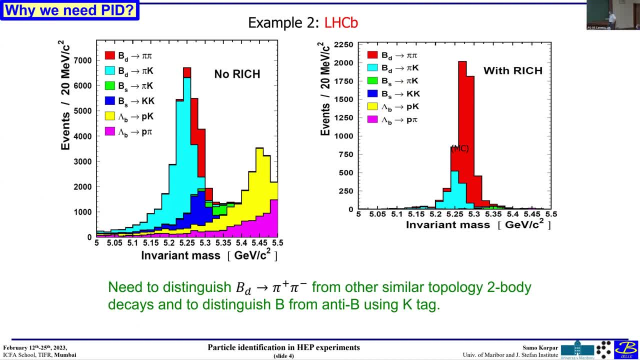 Be They look for, Let's say, B zero to pi pi Or pi k Decay, And you can see this Main peak Of these two decays And there is a lot of Background That comes from the decays. 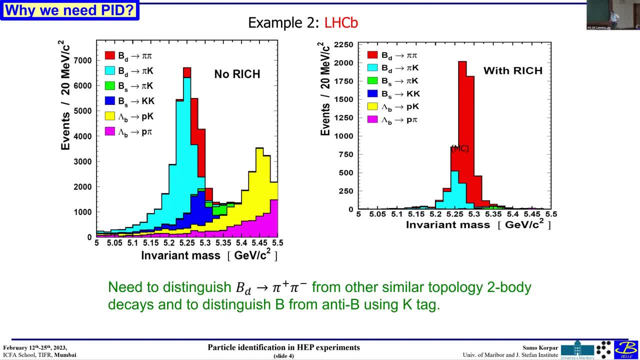 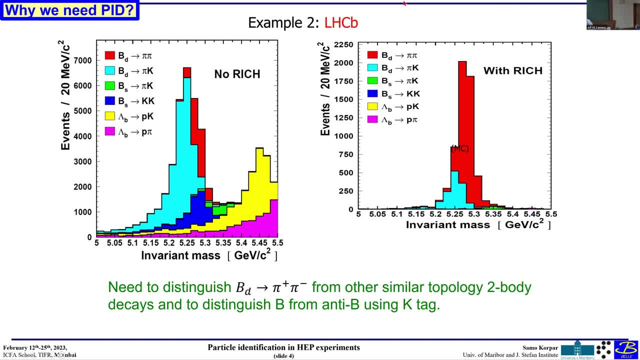 This one? Yeah, No, There's one, No, Okay, Oh, Everything is hidden. Okay, So You can see Basically That after Applying The Proper Particle ID, The nicely The search Decay. 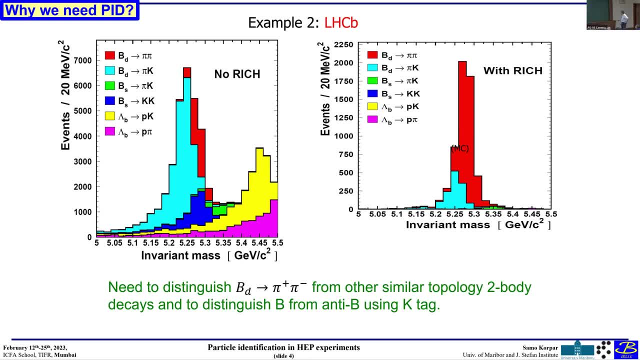 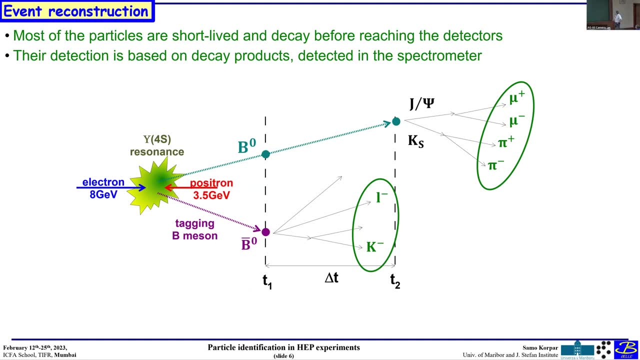 Sticks out And all The backgrounds rest. Okay, I have to put it in focus. So now, as I said before, we actually do the collision and then we get the decay product. some of them are short-lived. This is so-called. 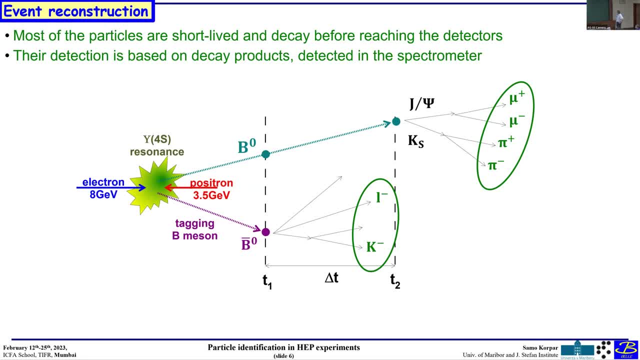 golden event at Bell or B factories to study CP violation in the B system, And in this case you get epsilon resonance and then for S, and then you get two B mesons, B and anti-B, that decay further And at the end you get the particles green here and green here. that 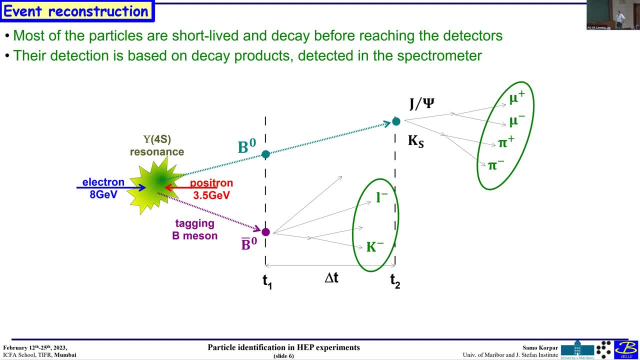 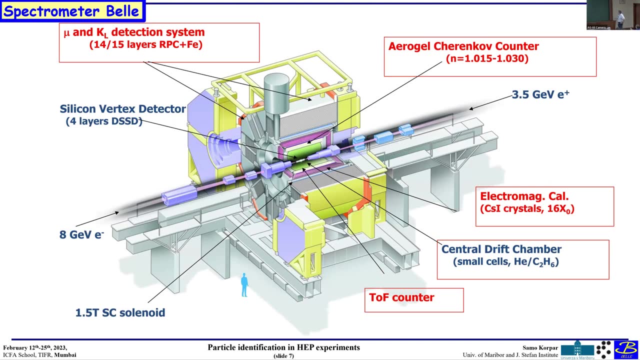 actually interact with your detector. So there are only few kind of species- we will see the table later- that interact and you have to measure any identify or separate between these two species. Now, typical experiment: I choose Bell because also quite few slides will be on this topic, So you can see you have usually a tracking. 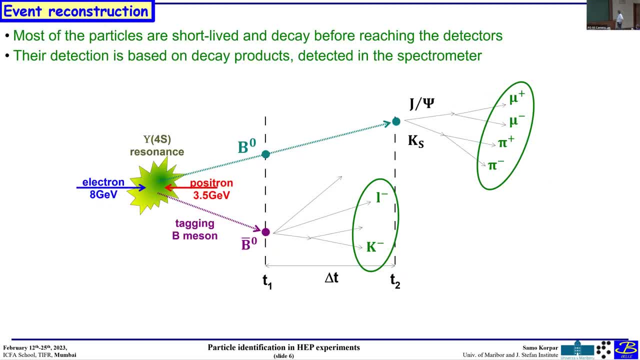 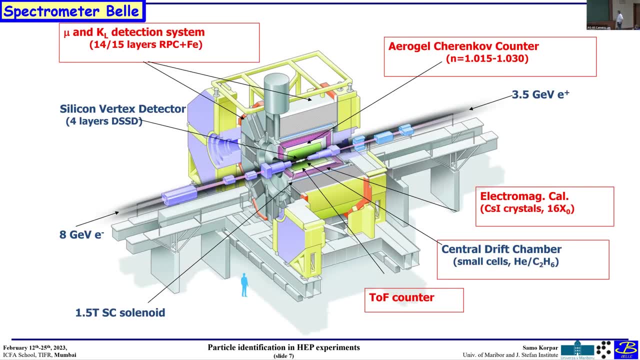 a very precise tracking inside and then more coarse tracking in this type of, let's say, drift chamber, which is also used then to measure specific ionization and to do some particle identification. Electromagnetic allerometer can also help identifying particles. also detects neutral charged or electromagnetic. 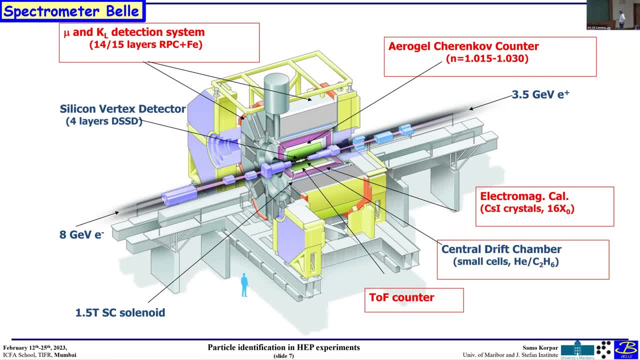 interrupting particles. Then there is a time-of-flight counter, which is dedicated PID device, aerogel threshold sharing code detector- basically that is around here- which is also dedicated for particle ID, And on the outside you have basically outside. 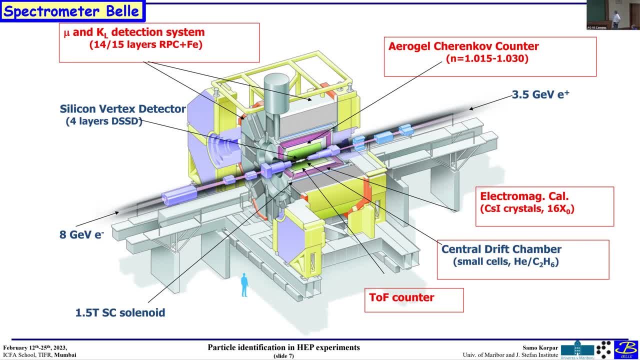 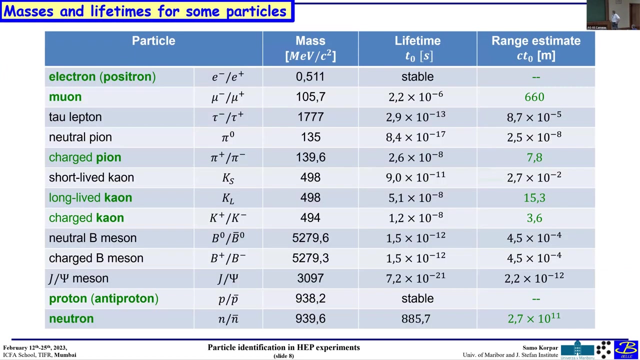 the magnet yoke you have a detector that basically detects neurons, that penetrates through all the other detectors and leave the traces there, And it's also basically a sampling hadron colorimeter to detect neutral long-lived K mesons. So this is also part of the identification in the detector. 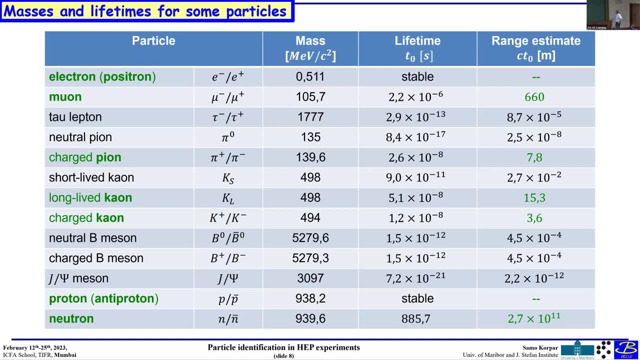 Here is the list, basically, of some particle, the ones that basically were shown before, and these green ones are long-lived enough to leave the trace in our detectors. So from the leptons there is electron and muon somewhere here directly, and this is the. 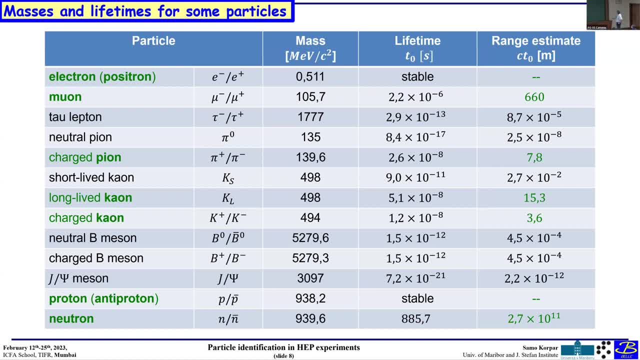 lifetime in the reference frame mass and this is the range estimate basically for beta gamma one. so just a lifetime times the speed of light and you can see that muons actually, before decaying to electron and neutrinos, they live long enough to travel very long distances. A charged pion. 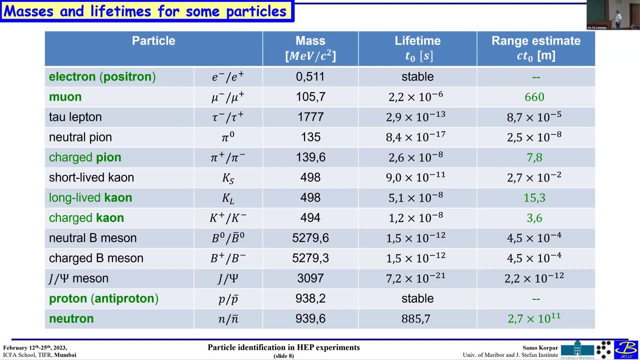 travels also long enough. far enough, long-lived neutral kaon, as we saw before, also lives long enough. Charged kaons live long enough to travel far. Proton, antiproton are stable, unless of course antiproton annihilates with a proton and neutron, basically antineutron. 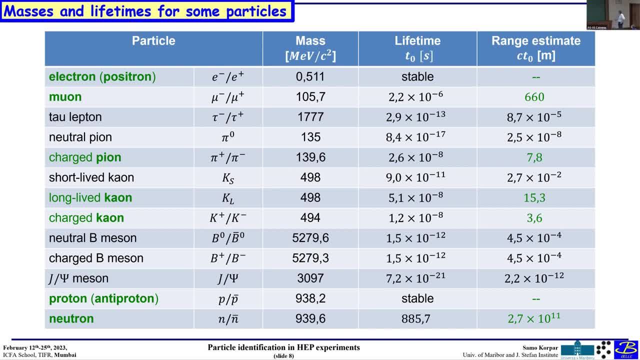 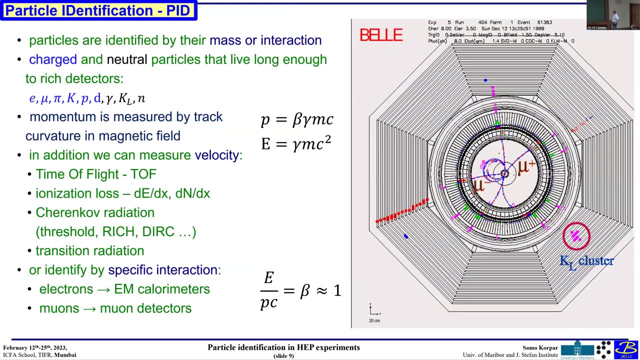 also live long enough to reach our detector. So these green ones directly leave the trace. all the others are basically identified or reconstructed with measuring these particles. So, as we said, they, since we only have a certain number of particles and they differ by discreetly, by mass, we can identify. basically. 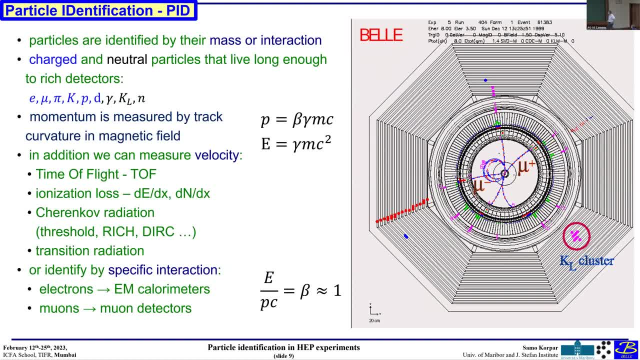 by measuring the mass of the particle somehow. So this is typically done for charged particles. The neutral particles are detected in colorimeters, as said before. So the charged are then only one, two, three, four. d is for neutron, which also emerges sometimes from our experiments. So you will see the traces of them. but 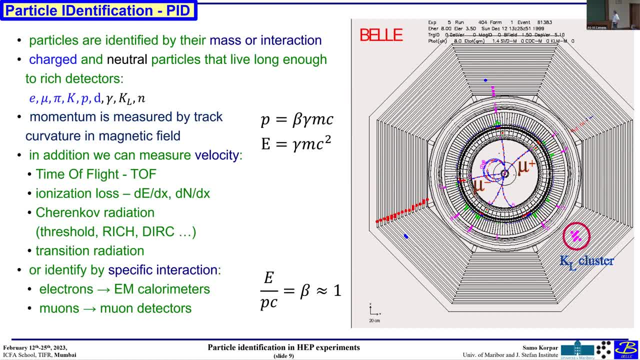 the first five are actually the ones that are the most important, And these are the formulas that we are all familiar with, relativistic formulas for momentum and energy. So momentum is measured, as we you know in the, by the curvature in the magnetic field that is present in the experiment. 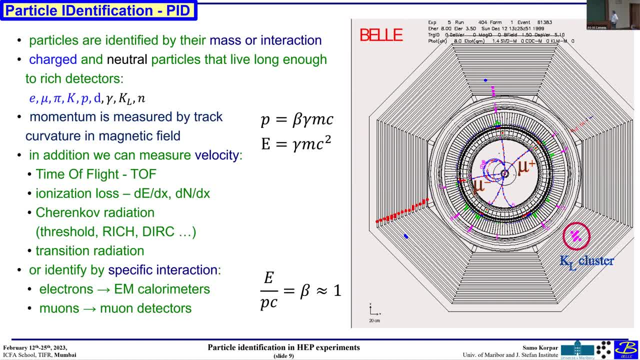 So this tracking system actually gives us the momentum of the mass. You can see that the mass is the particle and in addition then we can measure, let's say, velocity, and we will get the mass. and different ways to measure the velocity are time of flight. the simplest ionization loss is also 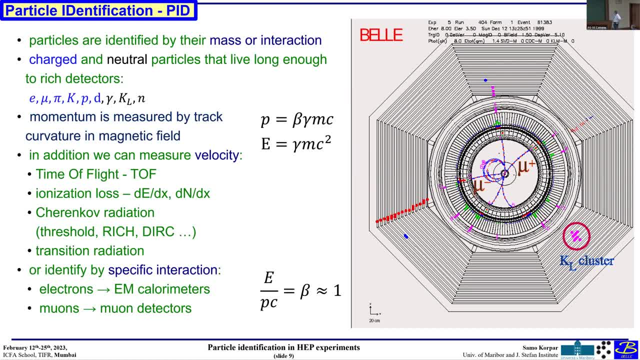 related to velocity of the particle. Cherenkov radiation is related to velocity of the particle and transition radiation to the gamma, so also to the to the velocity of the particle. so these detectors basically we will go through today is the plan to do all but Cherenkov detectors? 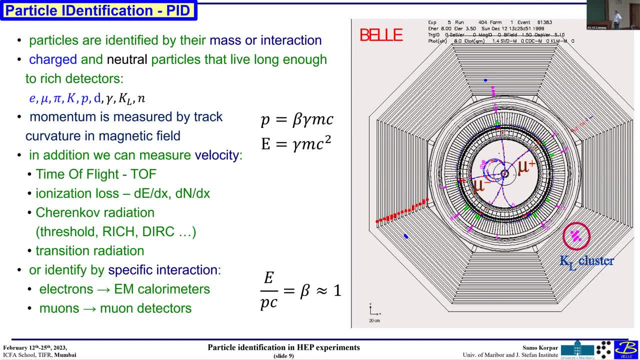 and then tomorrow focus on the Cherenkov based detectors. so some of the particles, others are identified by their specific interaction, let's say electrons, although they are also identified at high moment, very high momentum, by transition radiation. they are mostly identified in electromagnetism colorimeters. there will be special session on colorimeters so I will not talk anything about. 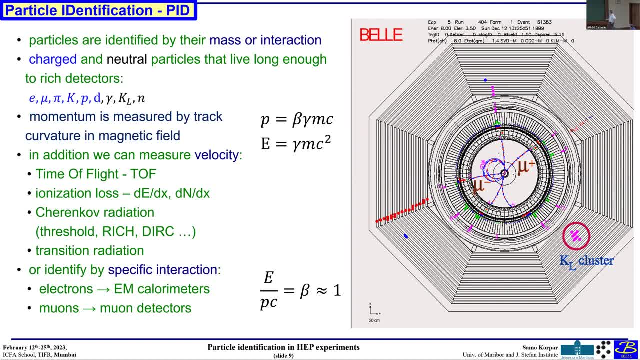 colorimeters. but simply because the they quite quickly the ratio between energy and momentum becomes one, so they are identified in by the this ratio in the colorimeters. muons, as we said, muons have actually a very high penetration power. they mostly lose energy by ionization loss. 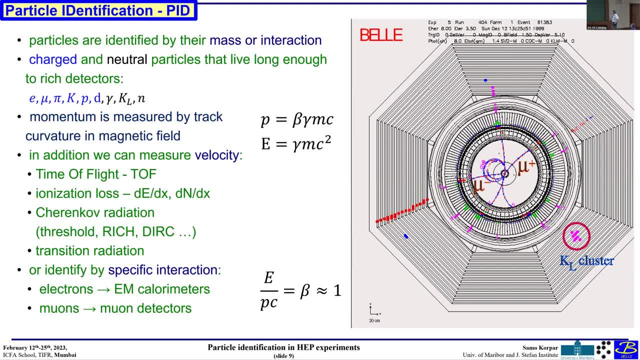 up to a very high momenta. so they travel toward the colorimeters and other detectors. you can see here a trace of muon, and then it goes out through the magnet. so then it bends then the other direction because the of course the field changes and you can see the trace of muon here. so this is 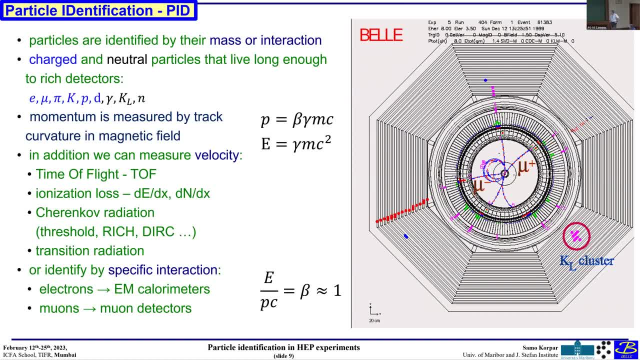 typically the way, at high enough momenta that muons are identified. at lower momenta they don't penetrate through, and in lower momenta other detectors try to penetrate to help with identification of muons. here also you can see that for neutral, neutral detectors, let's say gamma photons are detected in electromagnetic colorimeters and long-lived 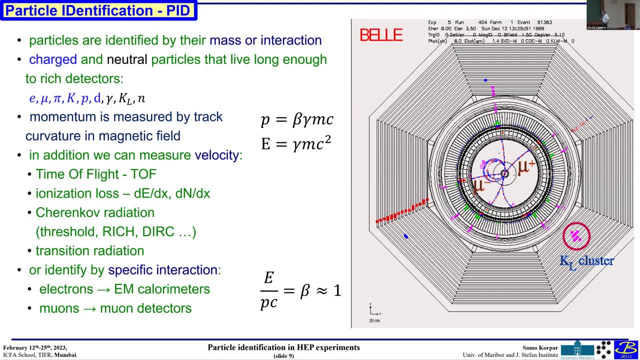 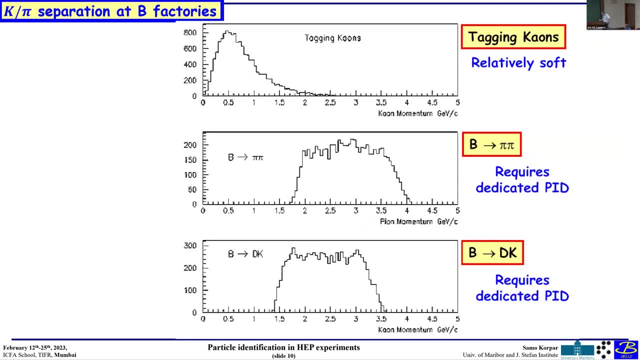 neutral kaon in hadronic colorimeter, basically in this case this outer detector which is combination of sampling colorimeter, hadronic and muon chambers. so these are typical identification techniques, and now let's look at one example how this is covered by different detectors. so usually most of the others are somehow covered. the main task usually remains. 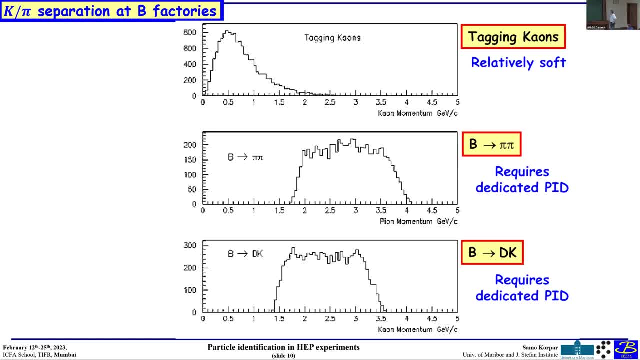 to separate kaons from pions in the detector. it is also true for the b factory experiment, where one of these was could be used for tagging of the flavor of the beamers zones and it was important to really properly identify kaon in such an event that was shown before. so their tagging 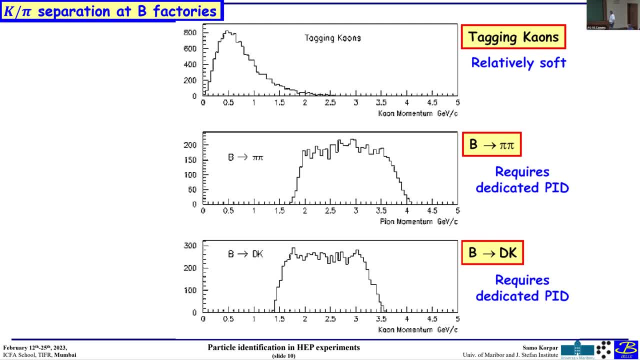 chaos are relatively soft. then we have two particle b decays, let's say pi? pi or k? k, that actually have a very high momentum and go in four pi around the similar decay beamers on to d and k and also covers high momenta a bit less because the mass of the d meson but also goes in all. 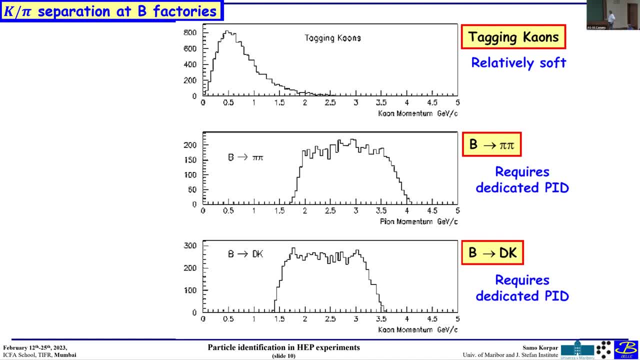 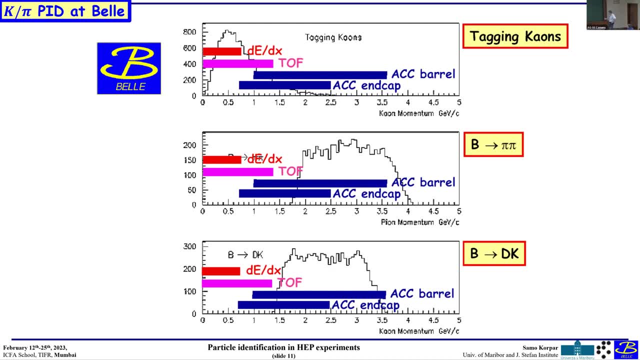 direction around in the detector. so there were two experiments, if you remember competing uh bell and babar, bail in japan, barber in united states, and two collaborations with the different detectors. so at bell, basically lower momentum, and also in babar, was covered by the specific ionization. 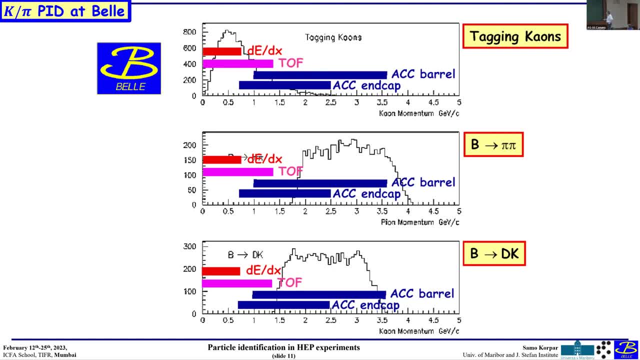 then bell had also time of light detector, which covered a little bit wider range, up to about- let's say one point, something we will see- momenta. and then there was a dedicated cherenko threshold chain, called detector, that covered the rest and it was optimized in around the beam pipe. 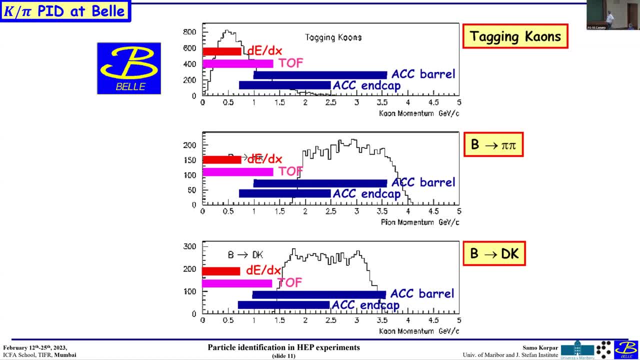 in the so-called barrel region, optimized to detect two particle decays, and in forward region, basically optimized to separate for tagging chaos. so this is a tagging chaos. you can see then the covering, the pi pi acc is mainly used and also for b2dk decays. 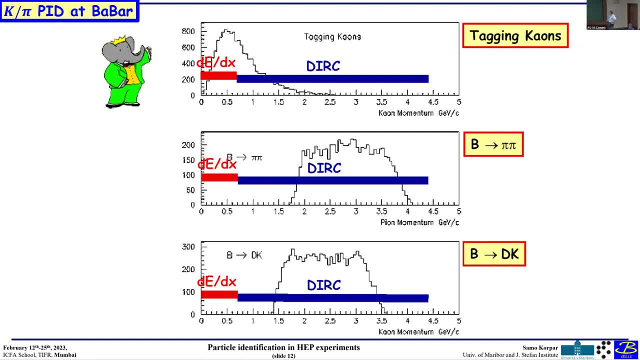 as we said in babar also, lower momentum was covered by the specific ionization measurement and for a specific particle id device they had a type of cherenko detector imaging with internal reflection, so detector of internally reflected cherenko light. we will talk tomorrow about it and in was covering basically the rest of the. 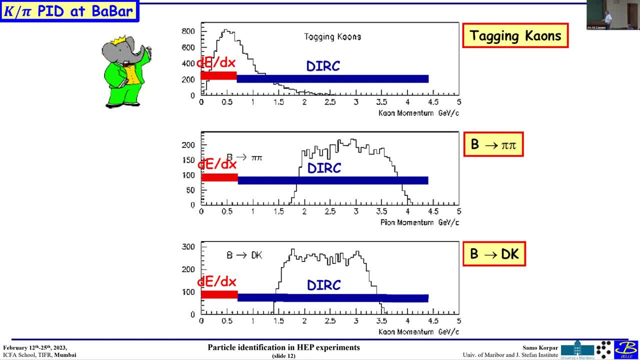 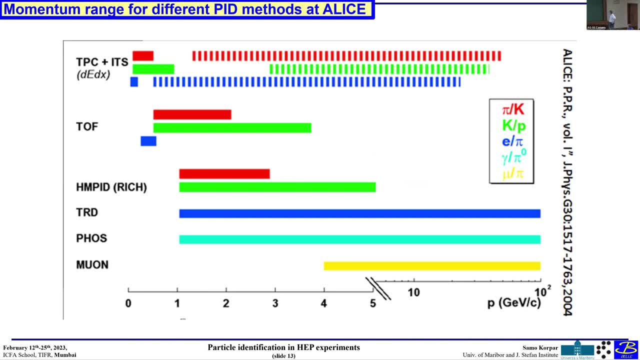 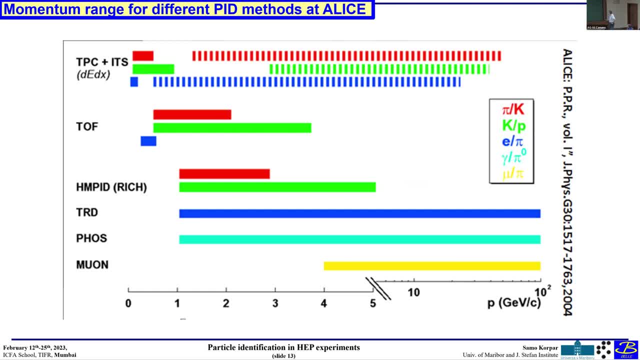 experiment and they basically employ more or less all the techniques. so they have ddx and different tracking devices. as we will see, the uh- a specific authorization- is good at low momenta and gives you some identification at higher momenta. time of flight. with bigger experiment they are longer. 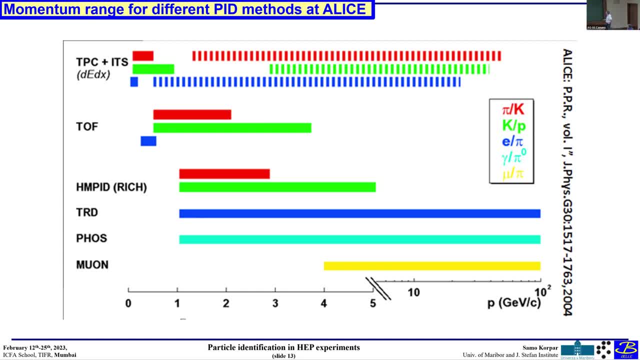 paths, travel paths, so it extends a bit to higher momenta. then there is a dedicated reach detector and transition radiation detector. this is colorimeter to identify, to detect basically neutrals- electro, electromagnetic colorimeter. and then there are of course neon chambers around to detect penetrating neurons. so this is roughly how the coverage of different identifications look. 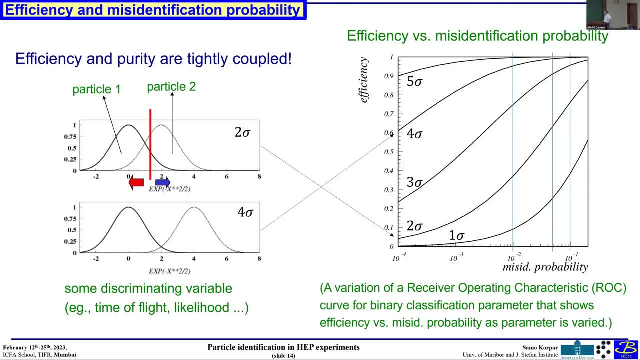 like in the experiment. and now just a few words about the somehow terminology that is used so typically we try to separate between two species of particles and, based on one parameter- whether it is time of flight or tedx or some likelihood calculated out of the distribution of heats in your detector- at the end we try to put everything down to one variable and let's say: 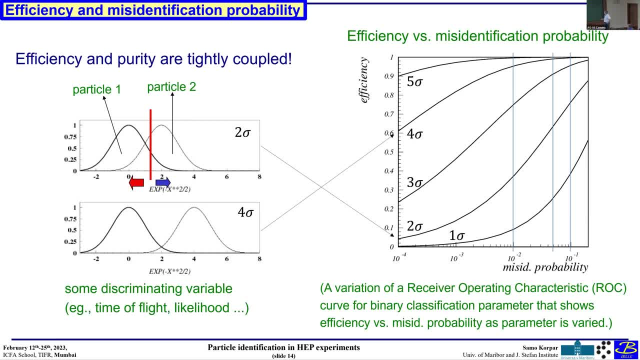 that this variable is gaussian shape, then what it means. if we say that the separation is two sigma, it means that the peak for one particle and the other is two sigma apart, and the how we define efficiency, the depends also on how much impurity we want from the other species. 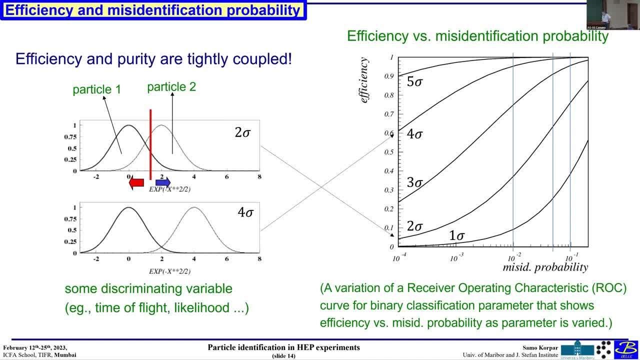 so we move this separation parameter, which is some sort of binary decision parameter, and there is a. if we move it one way or the other, then efficiency and misidentification, probability, which is this tail here, efficiency is this part here- changes somehow coherently. so you can see. 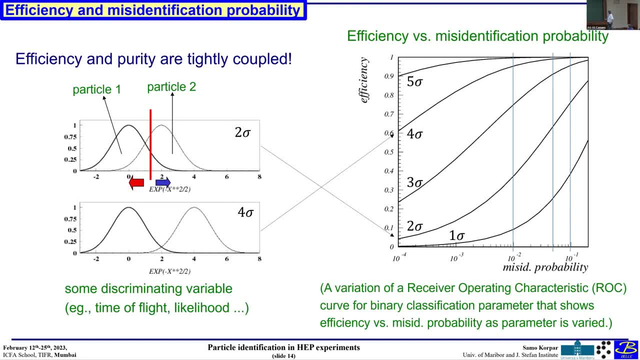 for two sigma separation. this is the line. this is the how much of the other species you get in your sample in percent and this is how much you properly identify. this is similar to basically the covet test. so one would be the properly identified sick people and these 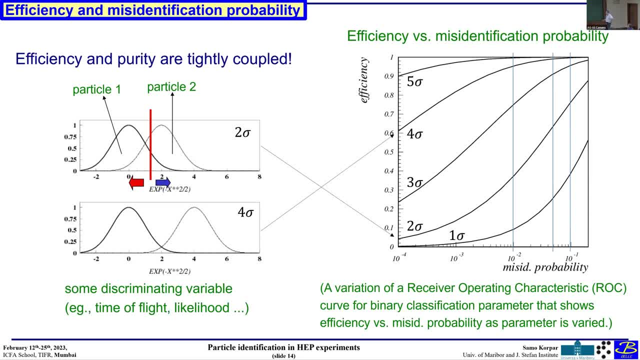 would be improperly identified, healthy people. so if we go to one percent of misidentification probability then we need about three sigma separation to come to about seventy percent efficiency and for sigma to go about ninety percent at ten percent. so let's say ten percent of the pions will. 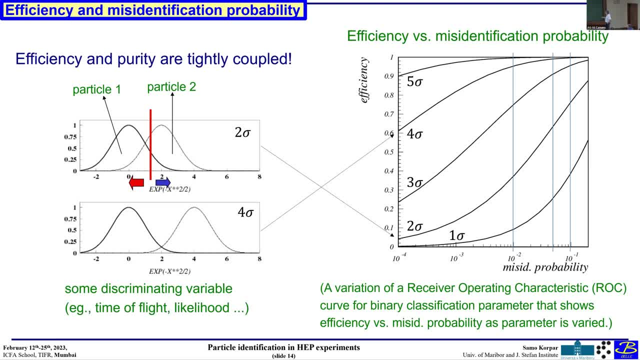 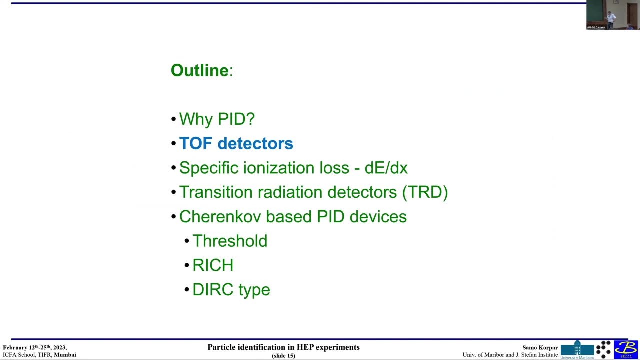 be identified as scales, then we will come with three sigma already, about ninety percent efficiency. so this is roughly what these sigma separations mean, even though they are not, then, at the end, gaussians. they roughly mean these fractions of the identified particles. yeah, now, that much about the general introduction, so we go now to the time of flight detectors. it's as i said. 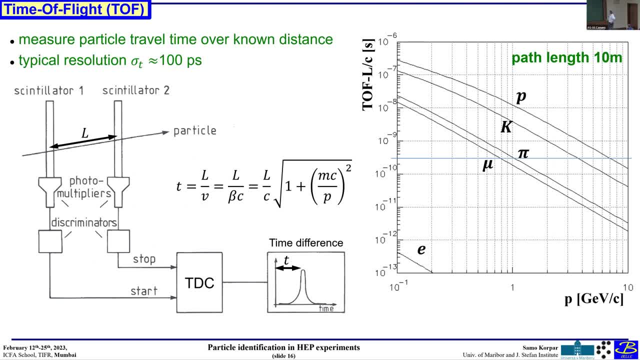 a rather simple concept. so we measure the particle travel time over known distance, like we used to measure the velocity in classical physics, typically schematically. this means that we have two detectors. that gives a precise timing. in this case, the same detectors, uh uh. nowadays in the experiment, actually, the first time comes from the interaction time. 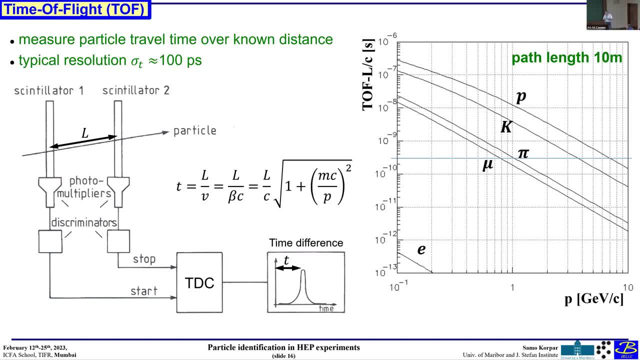 basically because most of the particle immediately decay and then these interaction times can be more precisely determined. so we only need one type of flight detector around then to make a difference. and then this difference depends on both how precisely we determine interaction time and how precisely we determine the particle. that 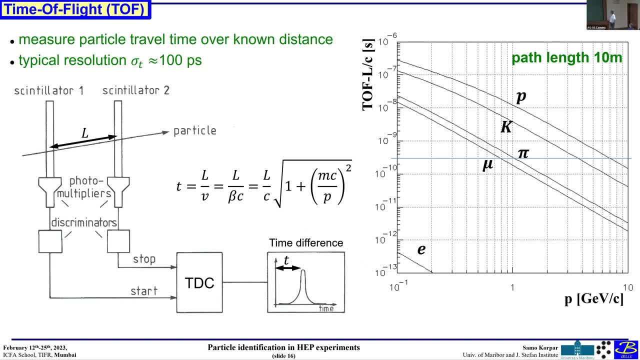 goes through our timing detector. so in this concept, basically, there is a length divided by velocity is the time that particle spends to travel this and this is related, of course, to beta of the particle and, at the end, to the momentum of the particle. so this is easy. 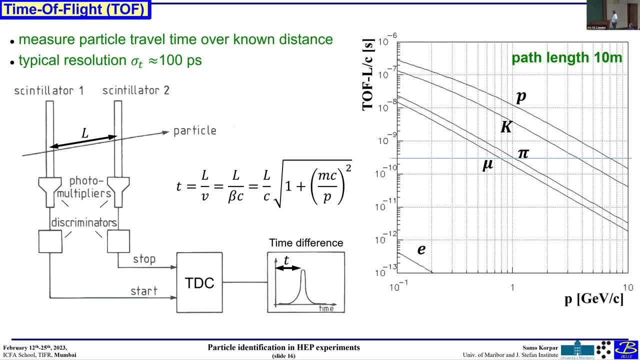 exercise for you to come up with these formulas. and if we plot this time now, you can see that basically it is a little bit larger but it goes. when the momentum goes up it goes to the, basically the time that light travels the distance. so in this graph the time of light is: 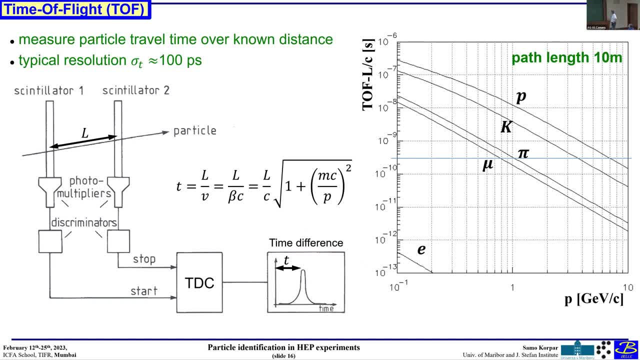 subtracted this light travel time and you can see what is the then the time at the different momenta. if the path length is 10 meter, this is typical for LHC experiments. let's say now, if we say that our resolution is around 100 picoseconds, 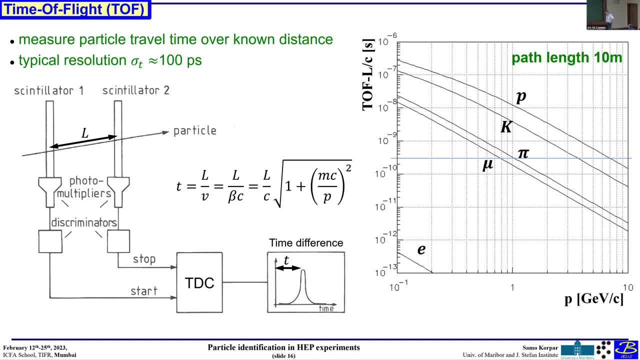 nowadays it's getting better. we are aiming at 10 picoseconds, but let's say at bell time it was around 100 picoseconds, and so to get three sigma separation we need 300 picoseconds- the timing difference between two species- and roughly this is just the 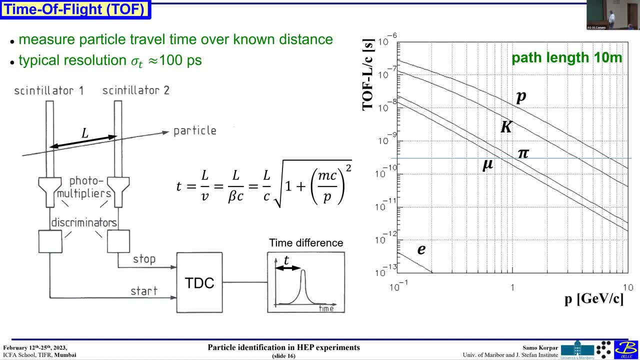 let's say, to separate kaon from pion. when the kaon reaches 300 picoseconds, pion is much faster, so that this is roughly than three sigma, and this happens about two, three and something gv at this path length. so the separation between chaos and pions. 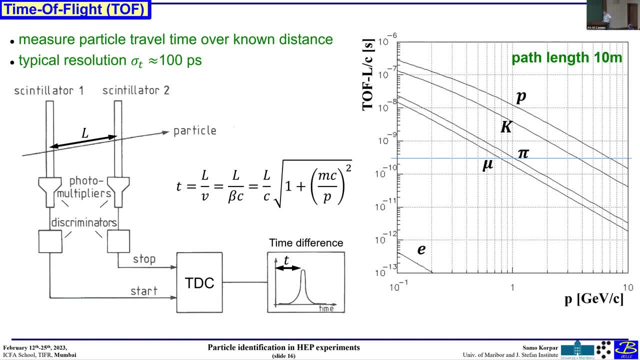 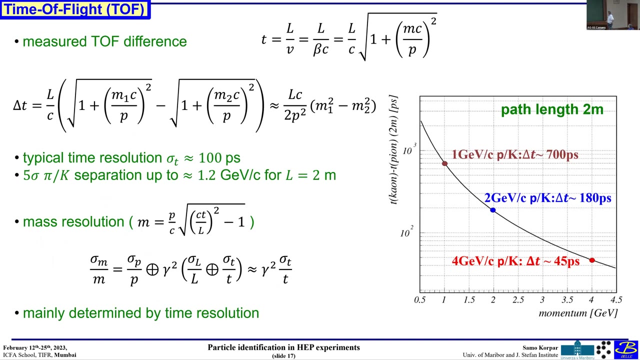 will be limited to about three gv. let's say, in such an experiment, if you measure in this way, of course, the total timing difference, the resolution is square root of two of the resolution of a single device. so what is the resolution where the difference between two times? is this simply the difference? 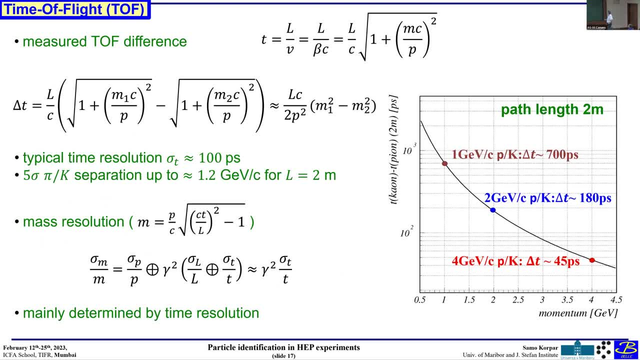 from the formula from the previous side and for higher momenta one can linearize this to this formula and you can see here the plot of the difference between pions and chaos at two meter length, more typical for smaller experiments. so at 2 gv the difference is already 180. 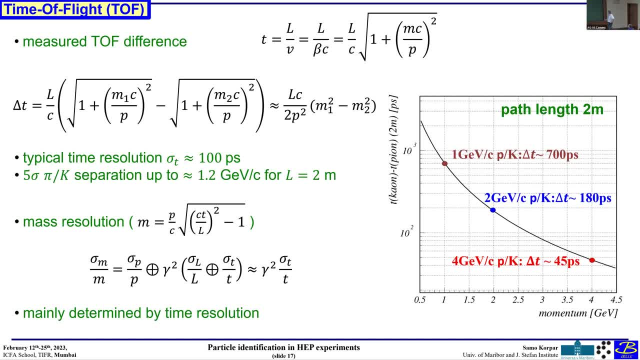 so one would need 60 picosecond detector for three sigma separation. at 4 gv it's 45 picoseconds, so really extremely fast detector would be needed, so in this range already. then the other cherenko techniques kick in at lower momenta, at one gv. 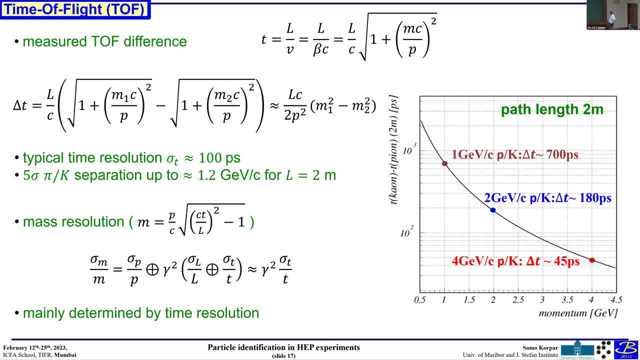 the difference is 700 picoseconds, which is more or less easily achievable by classical time-of-flight detectors. so, uh, resolution is then depends. here is written as a mass, which is finally what we want to discriminate. relative resolution of course depends on the track quality information, on the momentum, but 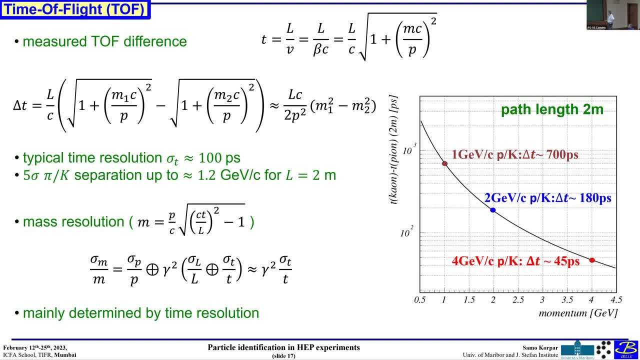 this is typically on the other one percent, so it's much smaller than the rest. then the other two: the length, which is also typically well defined, but at the end you actually have to take into account the curvature of the track and reconstruct the proper length, which is all then also burned with some 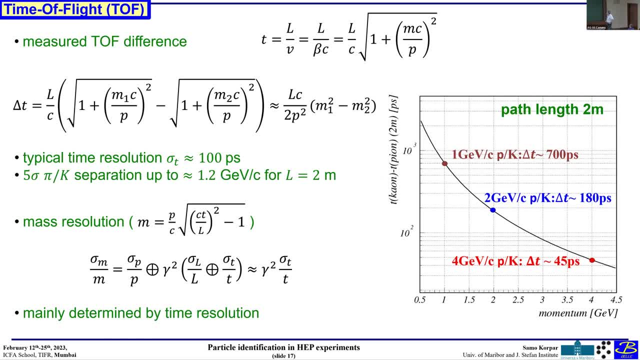 errors, but this is typically still below one percent. so the main contribution at the end is time resolution on the timing and these scales then with the lawrence factor. so at the end you really need a very precise timing detector. this is an example of bell time of flight scintillator. 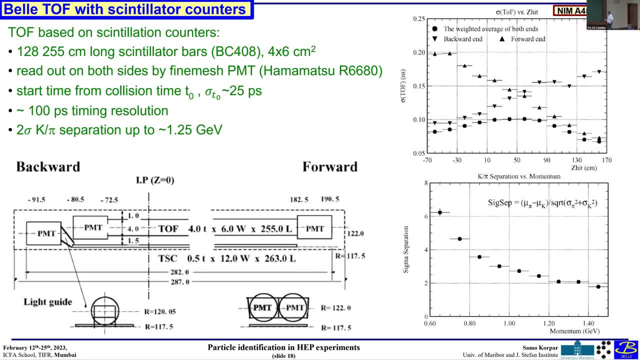 counter. so it was basically a 2.5 meter long plastic scintillator with a cross-section few by few centimeters, and it was read out by pmps on both ends. and these pmps we had to operate in magnetic field. so the fine mesh. 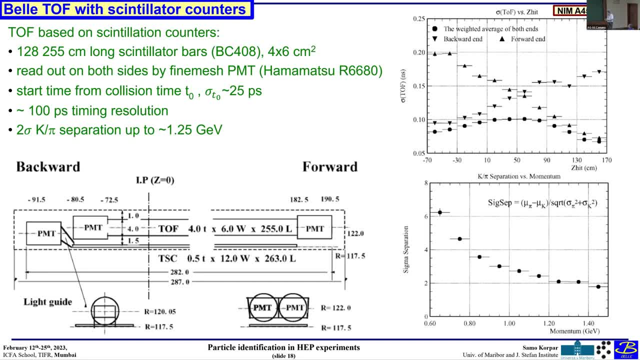 pmps. fine mesh means that the dyno structure is made of a metal mesh is used which can operate with reduced gain in the high magnetic field, and it also has a very nice timing: resolution on the order of 60 to 80 picoseconds, or very small. 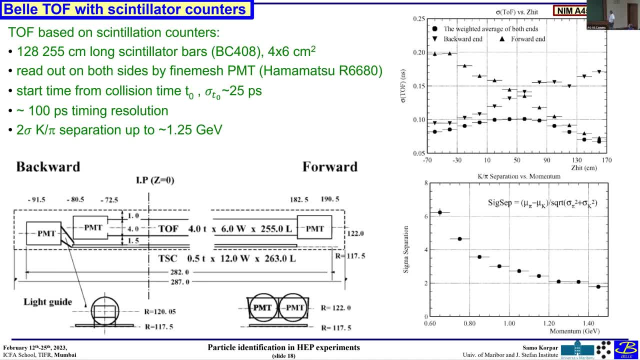 for single photon pulses. so the start time was defined by the interaction point. interaction time and was the timing achieved was around 25 picosecond. so the then the timing was defined by the time of flight precision of the scintillator detector, this upper bar actually here. 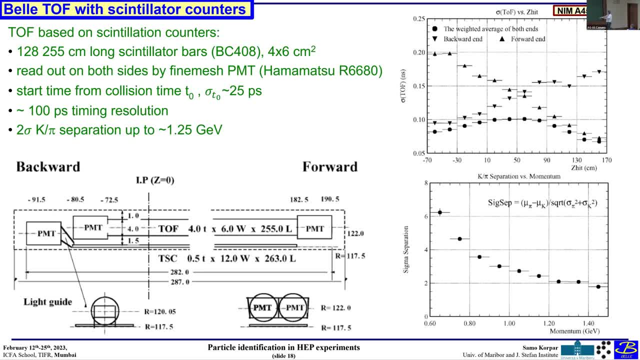 very thick scintillator to allow a lot of direct light with less reflections going to the pnts on both sides. of course the timing then on one side depends on the first of all scintillator, but this at this level is actually not really important. the decay time of the 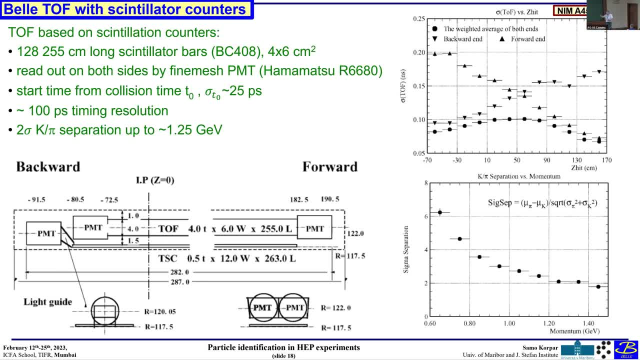 scintillator is typically on the order of few- now a few minutes, few, 10 nanoseconds. the plastic scintillator is on the order of two nanoseconds, and then the first photon. if it's only exponential, the first photon actually comes with a distribution that is shorter by 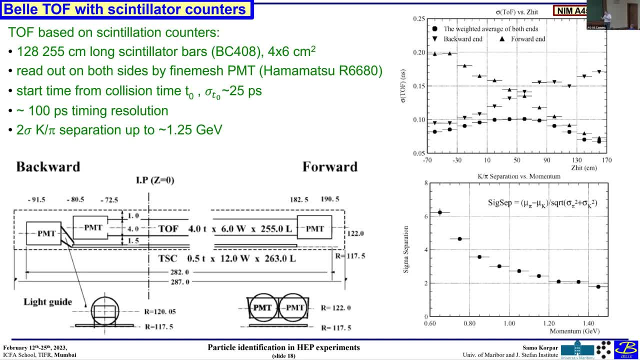 the number of detected photons. so if it's two nanoseconds and you detect 100 photons, in principle it would be. let me see, it would be 20 picoseconds if they would all straight decay and decay by exponential. that comes straight to you, but of course the main actually. 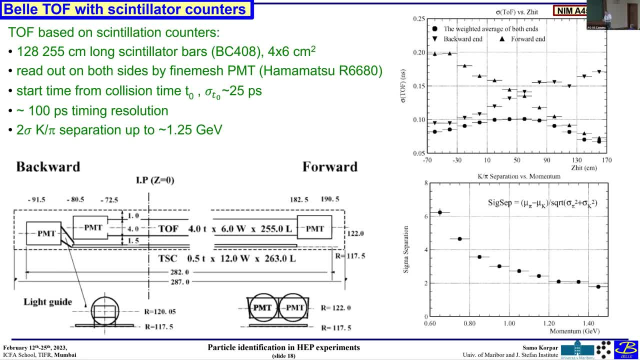 variation comes from the traveling of the photons inside the quarks and longer they travel, more in time they spread, worse, get the distribution. this you can see actually here. so this is the timing measuring on the left side as a position and you can see that it gets worse when the 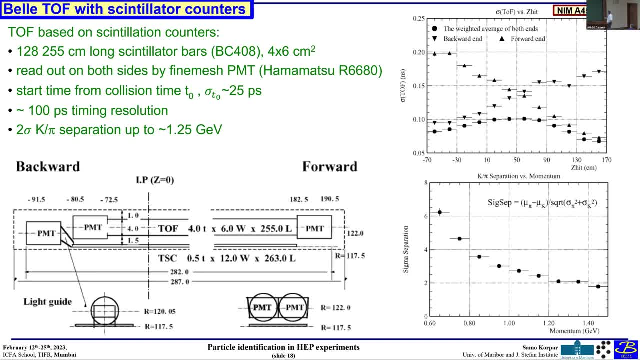 track goes to the other side, and this is the same for the other side, the pmt on the other side, and then, if you combine properly with proper weight, the timing, then you come all over to around 100 picoseconds or better in such a detector. so this was designed. 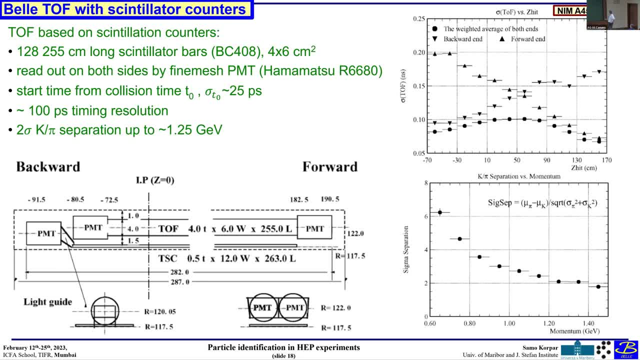 then to cover the pion and k on separation. even two sigma is not so bad. it covers the separation to sigma about to up to 1.25 gv and you can see the how many sigmas with the momentum it provides here. so two sigmas comes. 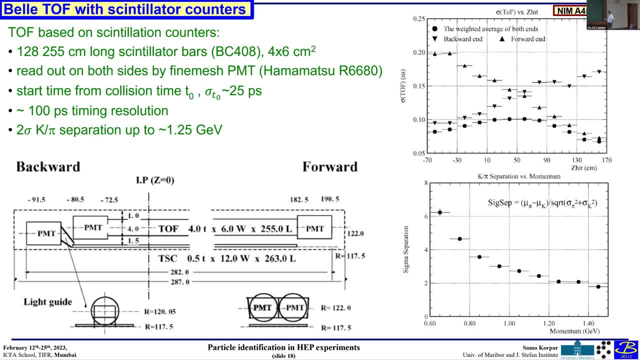 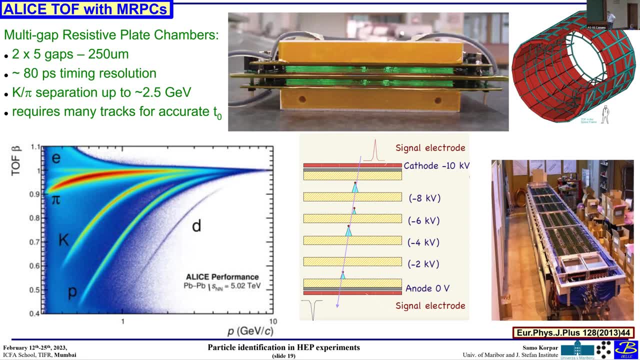 somewhere here in this region. yeah, so this is one example, the more the other possibilities nowadays, actually, several different material. this is the gaseous detector, the mrpc, so resistive, multi-layer, resistive plate chambers. you have the gaseous electrosome, gaseous. 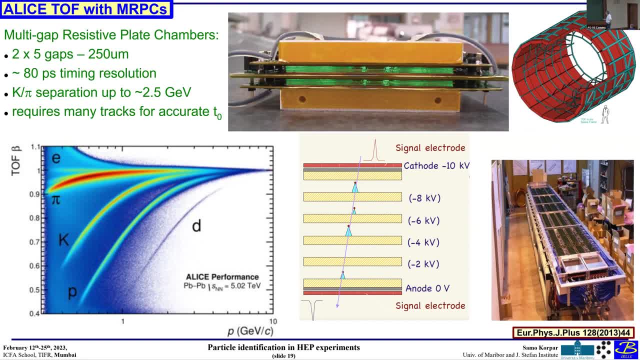 detector. so there are several gaps actually in between the high resistive glass which acts as an electrode, and then between there is a high field, linear field, and when the charge is deposited by ionization, by the track, this charge is amplified in one avalanche and then the signal actually is detected by only 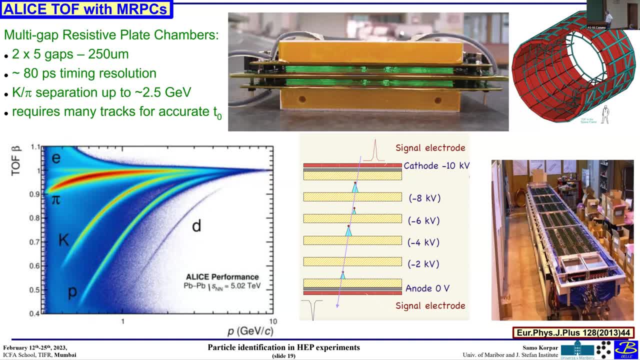 two electrodes. here you need to understand how the signal actually develops inside the detector. it's not that detected when the electrons come to the electrode, but all the time when the charge is moving inside the detector. there is induced charge on the electrode, so charge traveling from this point to 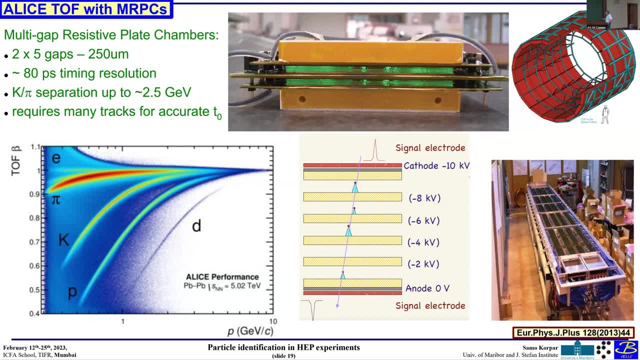 this point makes a certain pulse and then, of course, because these are high resistive plates, charge, stay there for some time. that stays there for some time and then diffuses slowly. so this part of the signal you don't see basically. so you'll see a very quick, fast signal. 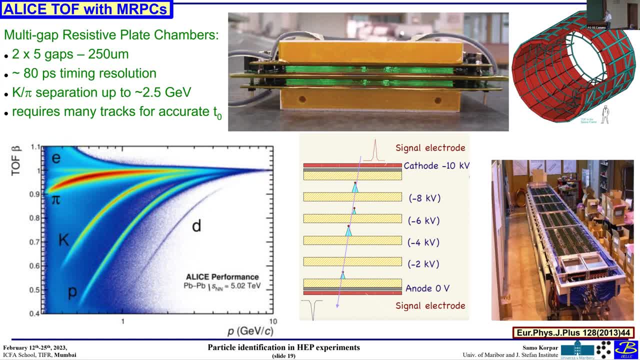 and because you have multi-layer sensors, then this is summed up and you have a larger signal, which is important for good timing, because the other contribution is of course the noise of electronics. and you, for really get a good timing, you need a very high gain multiplication factor in your 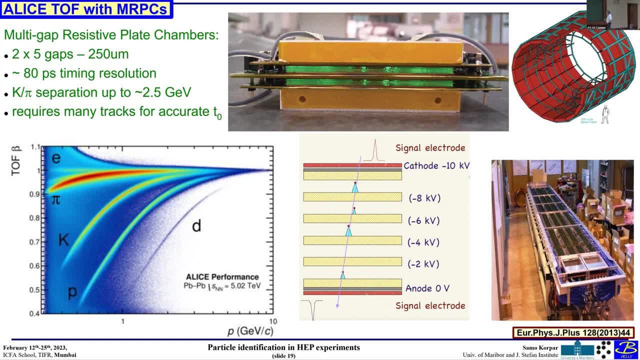 device a lot of signal. to really get a good timing out of your electronics with the low signals, you need to use longer shaping times, and then, of course, timing is immediately worse. so this is the concept and this is actually very far away from interaction port. there is a t0, again defined by the 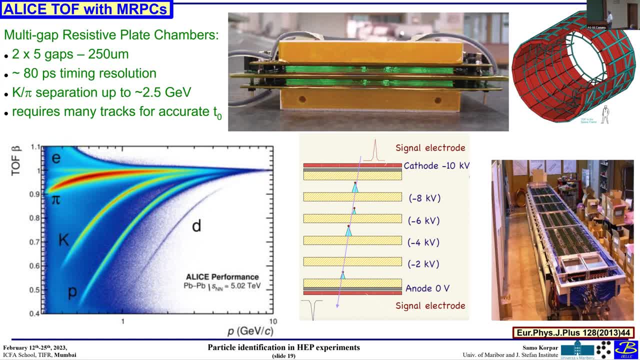 interaction inside and you can see, basically, time of flight, beta deduced from the time of flight, and this is momentum. and if you look at chaos and pions, you can see the separation, uh, let's say somewhere here which would be 2.5 or something like that. 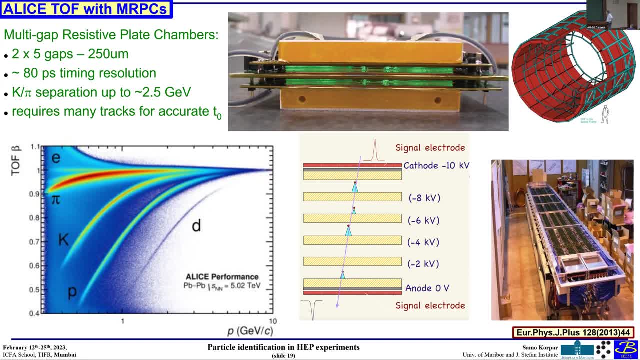 gv. here they become close to two sigma or something like that. so a longer path extends the identification and also faster detector. the timing of the end is 80 picoseconds or even better. uh, oops, uh, uh-huh. okay, there was another slide, but i afraid i 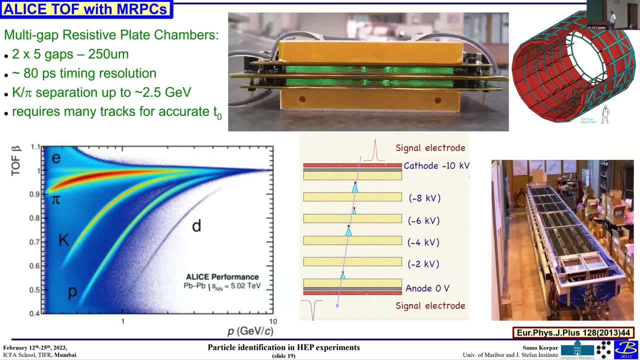 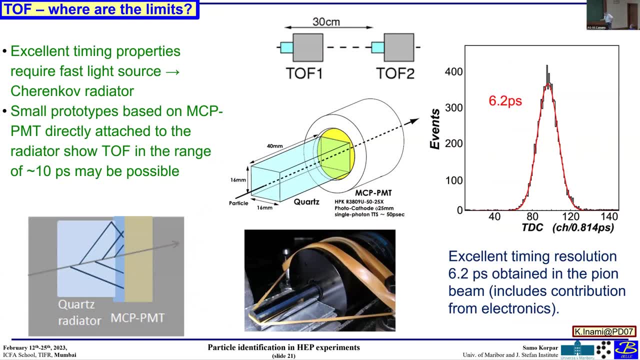 it is hidden. so, uh, no, it's better if i continue. so, uh, to finish with time of flight detectors. as i said, there are many different detectors nowadays that provide very bright, very fast interators, like, like, like lysol, with very fast photon detectors. the ultimate one, because the oldest, 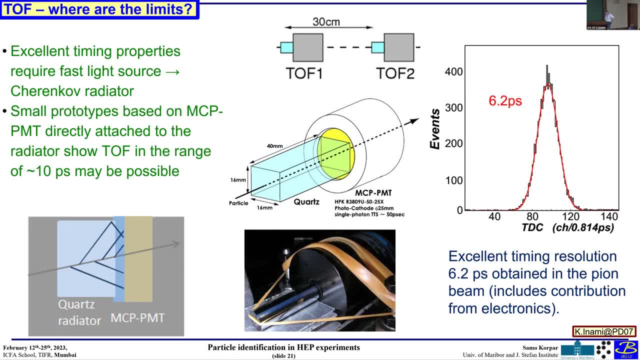 interlators have some decay time, but when you come to very precise timing, also the rise time of the scintillation light, because it becomes important when you have ionization- it's interlator first, the uh centers that then scintillate needs to be loaded and this takes on the order. 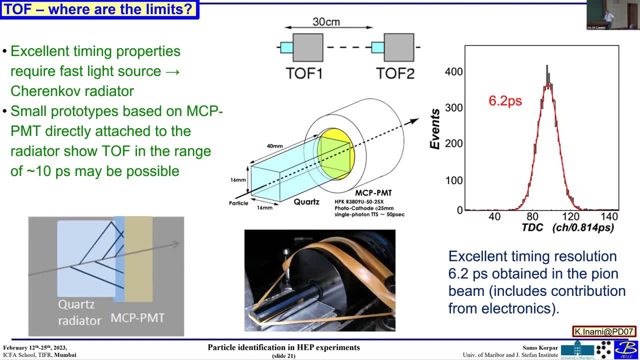 of about 100 picoseconds or so, and this already spoils the timing properties of scintillators, very fast timing so, in this sense, since the light produced by cherenko radiation, this comes a little bit in advance. i will discuss cherenko like later, but 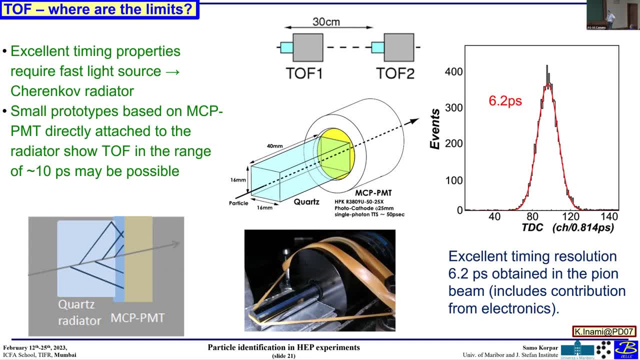 it's actually promptly produced by a very precise timing, and then it's produced when the particle goes through. there is no lonic and then decay time, and this makes it actually very fast. but of course, on the other hand, there is much less light. so if you go to extreme and then you 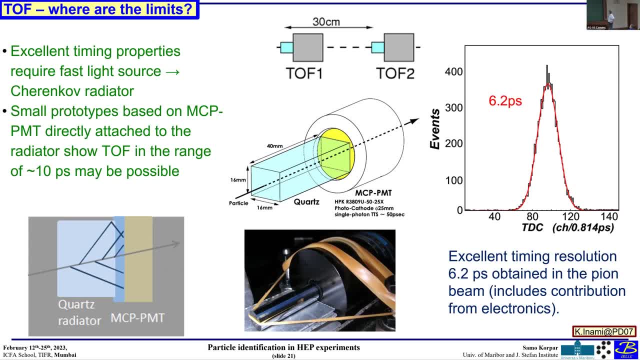 couple the cherenko radiator, let's say quartz glass, on top of the very fast photon detector mcppnt- we will discuss it also later- then you can get a lot of cherenko light, with a lot of light coming to your detector and putting two together actually. 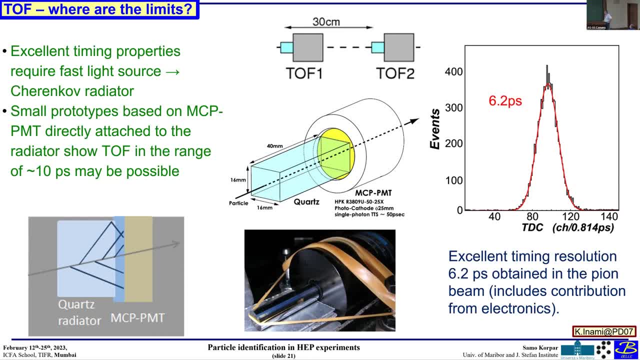 nagoya group measured the time of life precision of 6.2 picoseconds, including all the other contributions from electronics and so on. so one of possibilities is to go to the cherenko light. of course you cannot repeat this, at least now, at the moment, at a large experiment, so you 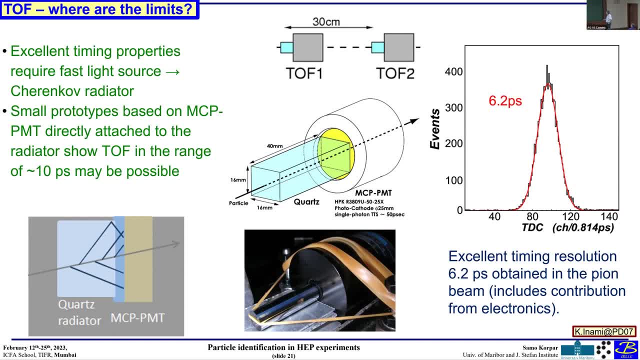 need some other techniques, as we will discuss tomorrow, but cherenko light is something, one of the things that can improved, and there are this low gain uh avalanche dials that are used nowadays introduced for tracking in high energy physics, that are also have a higher charge in silicon. 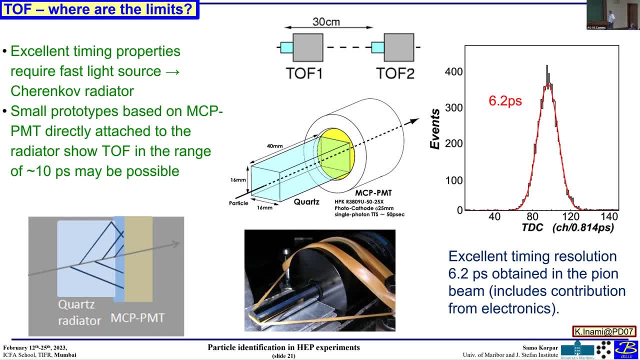 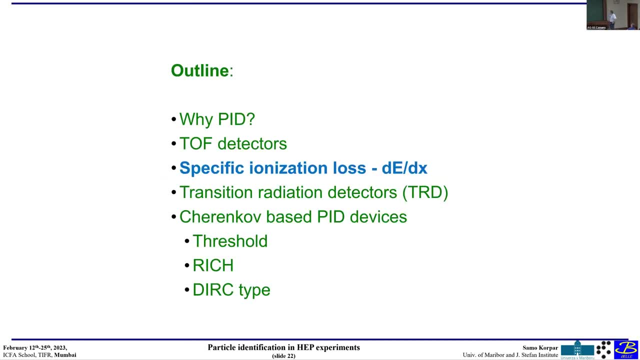 detectors that also can provide better timing than in addition to tracking. so several different possibilities and with this the time of flight extends slowly up to 10 gb, let's say at large experiments, but of course it will always be limited. so a short part about the specific organization. 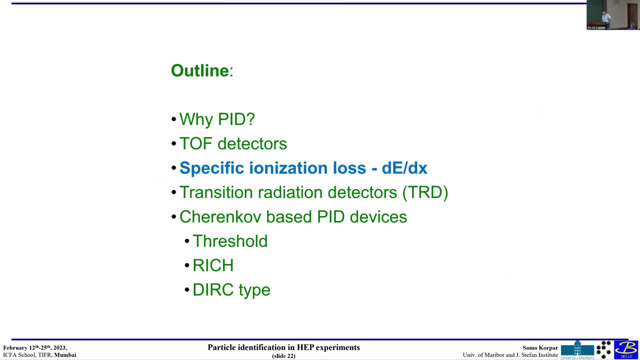 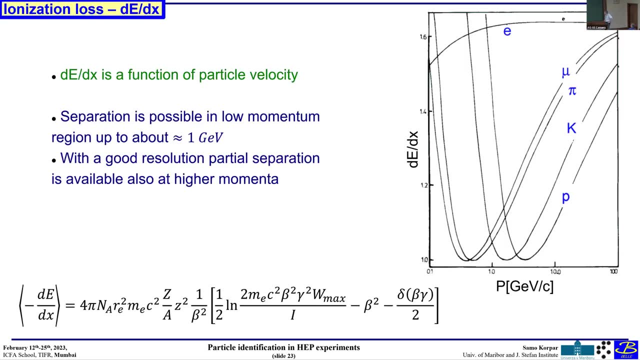 loss. this is usually part of the other tracking detector techniques, so it's only, uh, i would say a sort of a side product in tracking detectors. so this is beta block formula, as you remember. at least this first part, that it is for lower momentum, depends as one over square root of one. 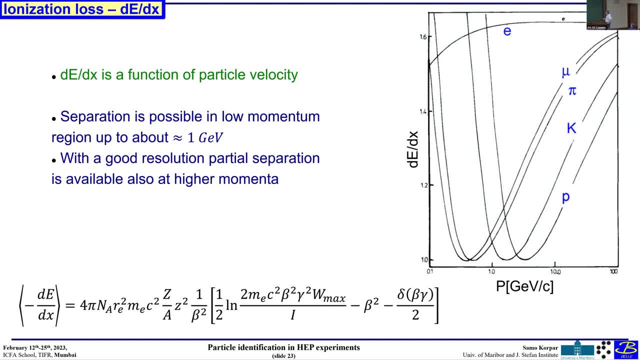 over square of uh velocity or beta, and this is this initial part here, and, of course, overall it depends on the velocity of the particle and at the same momentum, uh more massive particle have lower velocity and this is basically then shifted to the right, to the higher momenta. 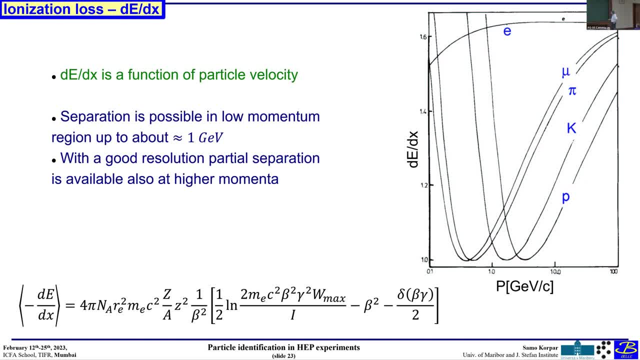 it is the same curve, roughly. so now what means the lower momentum, up to somewhere about half a gv? uh, this curve hits the minimum and then this part, uh relativistic rise kicks in and uh, you can see that then actually this uh specific organization for different particles overlap in certain regions. so 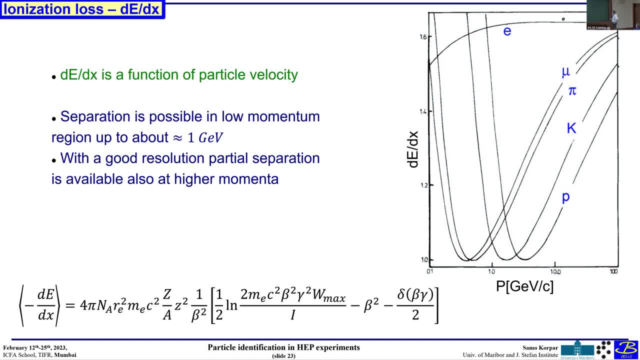 this is, let's say, pion and this is kaon. so in this region around one gv they overlap, so there is no separation in this region. then they hey, there is a rise where there are still apart. but you need a really good resolution to achieve, let's say, two sigma separation. 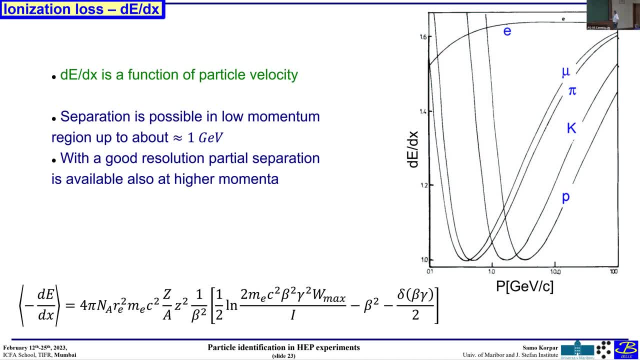 in this region. that's why in this lower momentum below alpha gv, dedx provides a very good particle separation. there is a kind of a dead region, and then about that region, about one gv or so, you still again start to get some separation from uh specific ionization in. 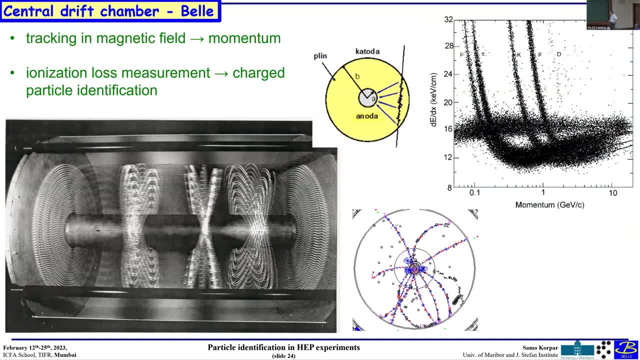 the devices. so this is an example: uh, uh, tracking. uh, basically, this is the, the central drift chamber, cdc, called at bell experiment. uh, there is a large gaseous volumes and then there are several wires, the thin ones that are to amplify and collect signals, and the 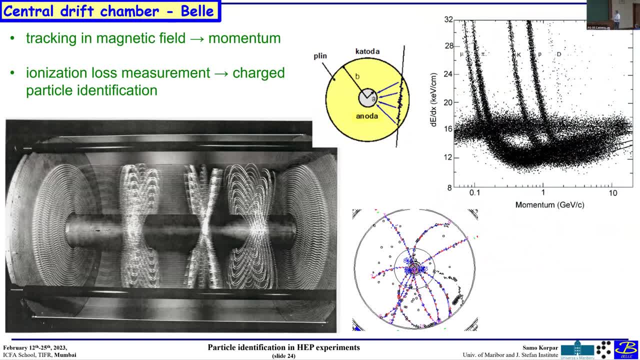 thicker ones that actually make the cell structure in there and because they are also at three different angles to allow have the position measurement in this direction. you can see these three kind of disc reflections in here. so there is a lot of wires and each set of wires forms a cell. 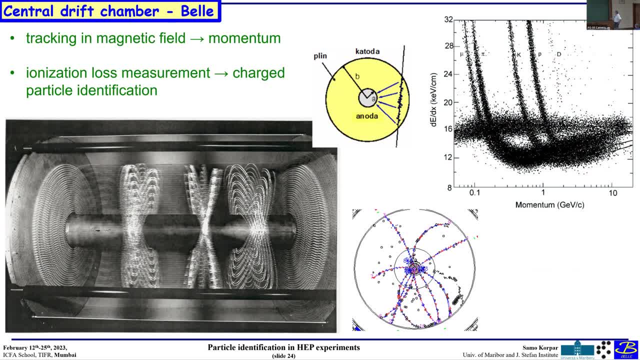 just schematically plot here and when the particle goes through, you get this specific ionization and then this actually is collected. the timing gives you the more proper position and the amount of charge actually combined from several cells. you can see a lot of cells in the particle track combining the 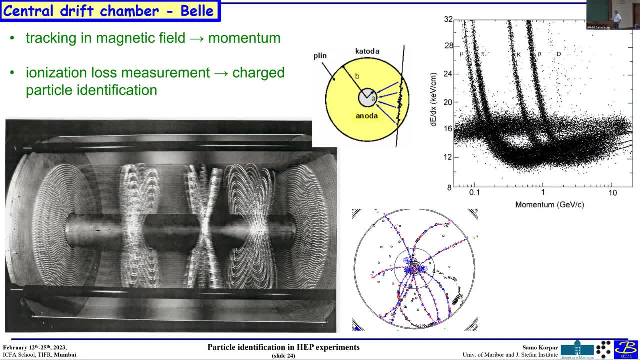 charge from a lot of cells then gives you, and averaging gives you the average d, the x, and you can see then for pion k on, as we saw before, somewhere up to half a gv or a bit more. there is a good separation and then there is no separation here. 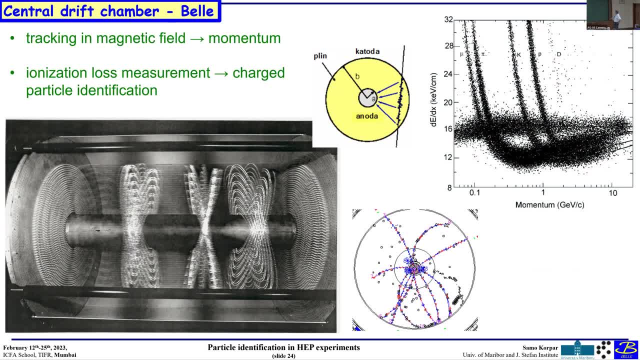 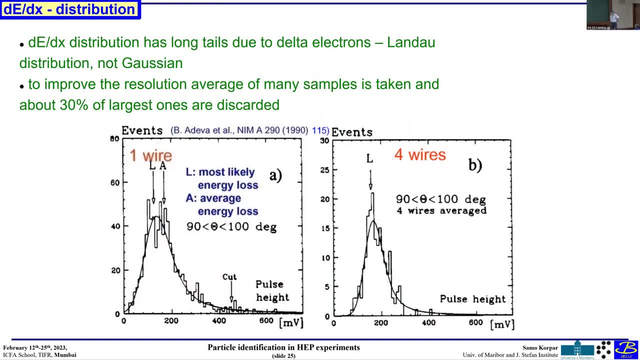 and then they again split a little bit in this region, not very well seen on this plot, and then you can see that this is a very specific ionization. now, this specific organization, you know that it's not basically very, all, very low momentum electrons. they have a certain spectra and there are 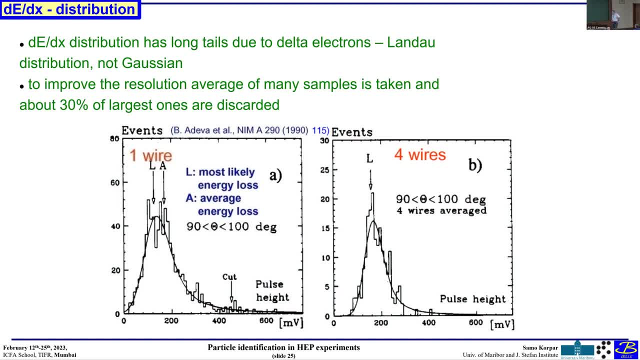 some with very high: 10 kilo, 100 kilo or even more- energy electrons are kicked out of the material and this produces- if you look at the one wire spectrum, of course this is the average. somehow of that you have sometimes a very energetic electrons, delta electrons, that 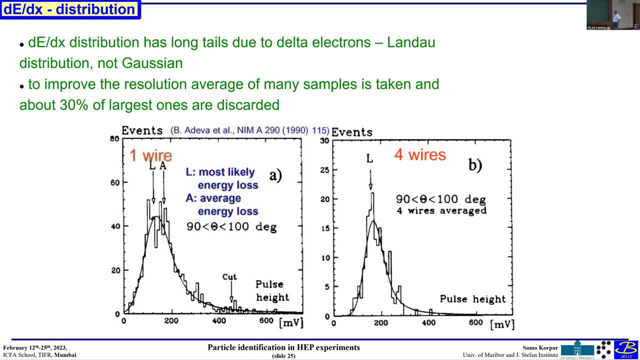 are kicked out of the material and they produce a very long tail which then, when you do the average, makes a very high fluctuation fluctuations. and to reduce this, basically, what is typically done is to make average so the in a way that you discard, let's say, 30 percent of the. 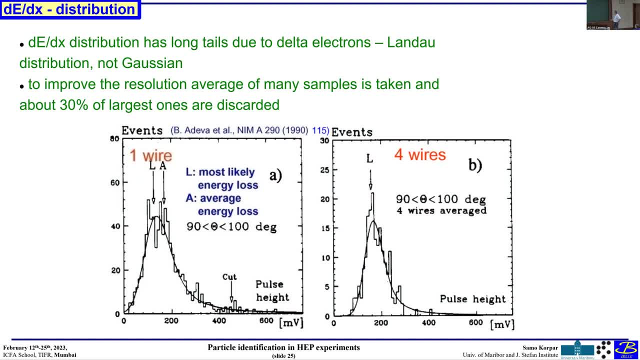 largest, largest heats, you make a cut and then you make the average of the rest to get a better separation or better resolution. so this comes then from four wires, and then so on. you have a several wires, 50 layers or so, so you get the resolution down to few. 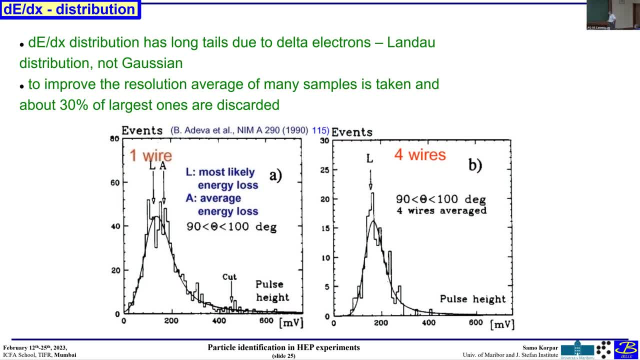 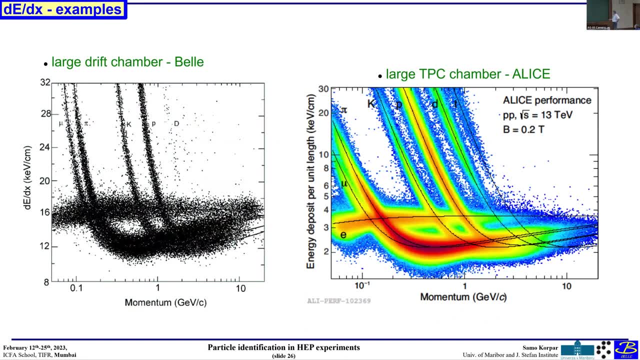 percent. typically in such detectors these are. this is already the example that i showed before. this is the large drift chamber where the each cell is separated either in some kind of cylindrical structure or by the field wires, as the case in the bell detector. this is the large. 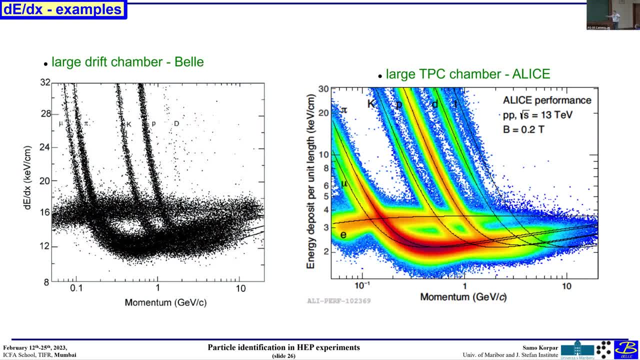 time projection chamber. this is the large volume. you probably had it in gases detector, large volume with a constant field when the truck goes through. actually, the charges drift down to the your detector, wire detector and from the time you get the position and from the charge measure, the 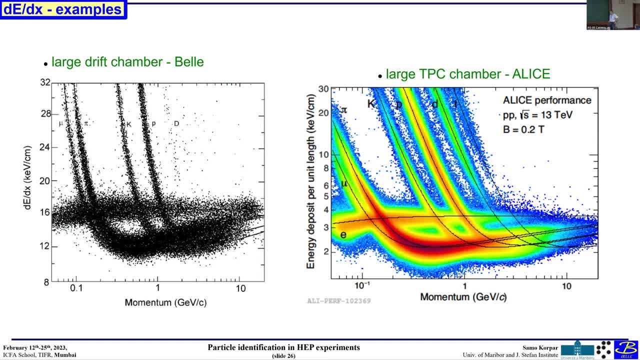 different points. you again get the samples of the dedx along your time track, you do the averaging and then you get the similar plot as here. this is the alice, a larger experiment as i showed before at lhc time projection chamber, which is used for tracking and also for 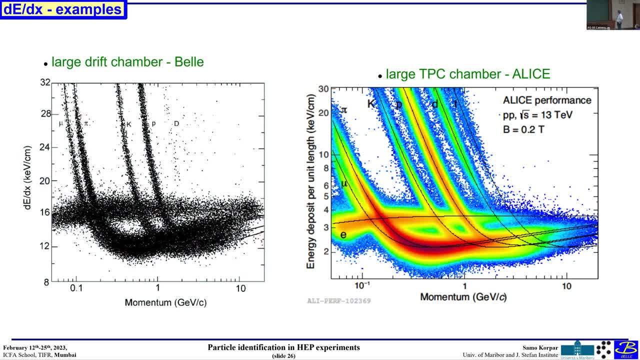 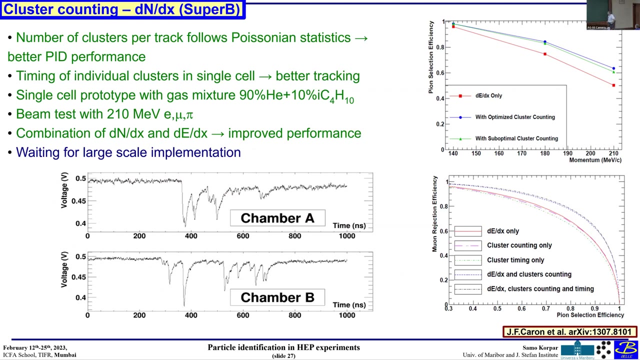 dedx. so pion again and kaon again meet somewhere about one gv and then after that pion goes here and kaon goes here. so there is some separation here. but the depends very much on how well the resolution is done. typically there is a chance to slightly improve. 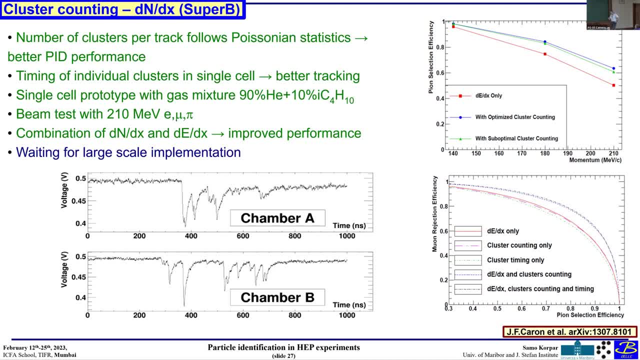 the resolution, because there are two things actually in the interaction. one is how many times the electron is kicked out of the material, and this follows the poisson statistics, and the other one is how much charge is deposited, and this has the tail because of the delta electrons, high energetic. 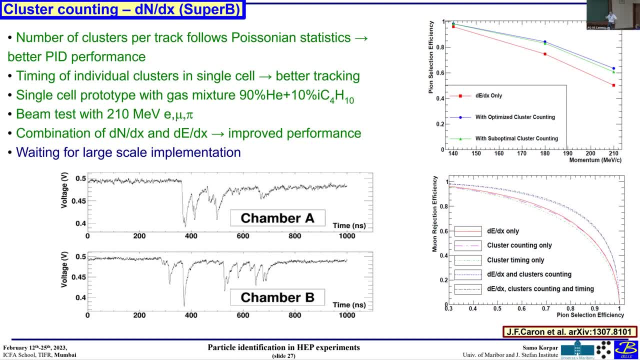 electrons. so in principle it would be much better if you would be able to count how many electrons were kicked out. then you would get a nice poissonian statistics along the track. but this is not usually possible and there were several attempts through the years and i 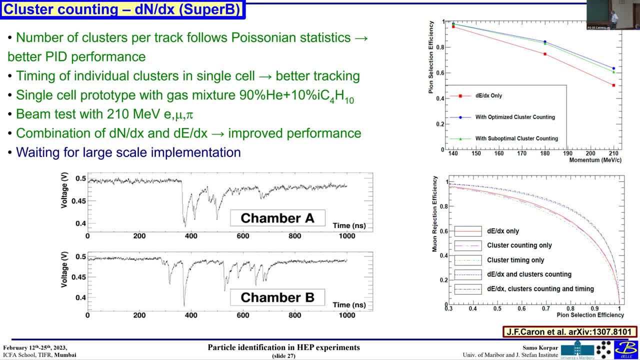 haven't seen the this really implemented. so the last one that i saw was for super b. this was the detector that would in principle succeed the babar experiment, but it was then cancelled. but they actually started the performance. so if you look at the drift chamber in one cell. 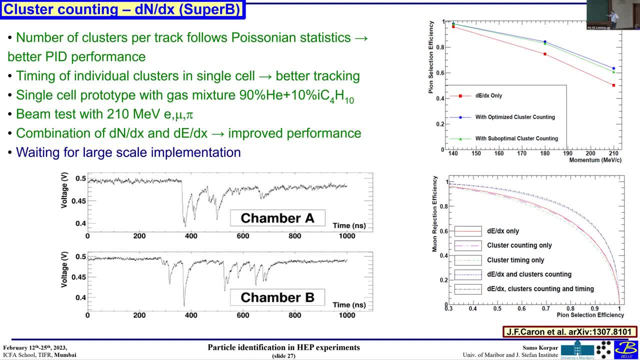 then the charges deposited drift over your anode and because they come in a kind of discrete way as they were produced along the track, they produce basically separate pulses and if you make the waveform sampler so that you actually measure the pulse height versus time, you could count how many. 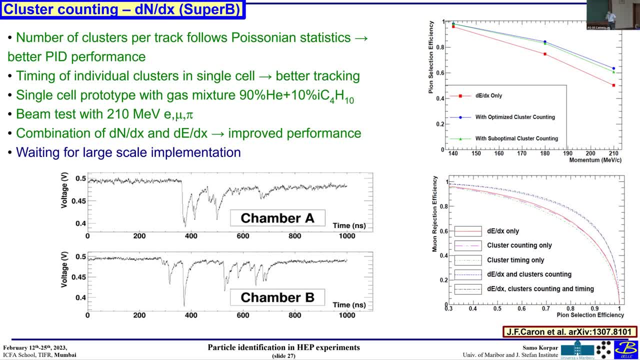 pulses you got, so you would get some information on how many ionizations were there, not only the amount of charge. and now let's say, just to look at this plot, muon rejection efficiency without using this cluster number information, this red line, and reducing the cluster information, a. 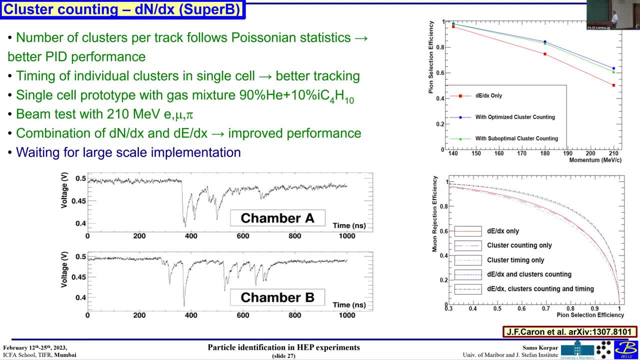 bit more of muons are rejected, let's say, as not being pions or in this experiment or in this test. so there is a slight possibility to improve, but it's probably much more work than it's actually worth at the end. so it's at the moment not really implemented. 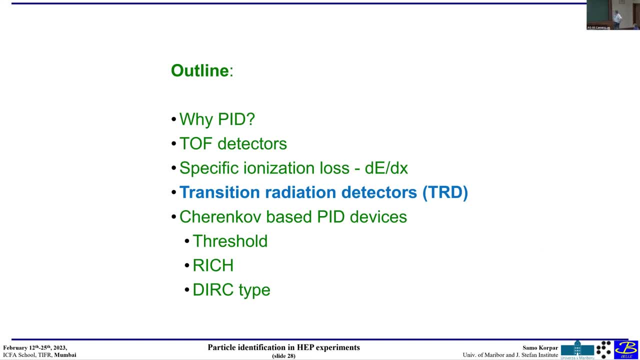 so these are the first two techniques, and then there is a transition radiation detectors. these two are actually, as we have seen, for lower momenta, so the time of light goes up to one gv, two gv with longer flight paths, more precise detector, maybe it will go to 10. 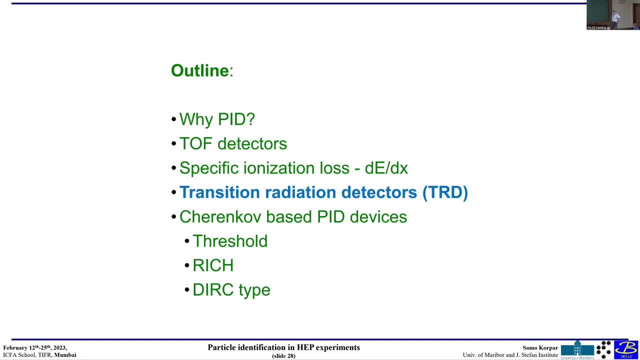 gv in 10 meters and 10 picosecond resolution. specific ionization covers up to, let's say, half a gv, and then there is a gap, and then it gives some identification about, let's say, 1.5 or 2 gv. uh, then there is a a very high momentum. 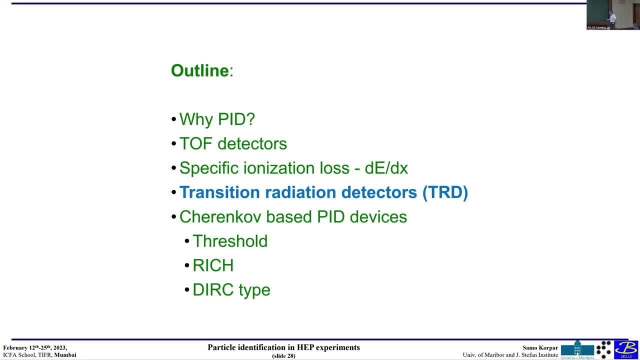 basically for electrons, one can use transition radiation detectors. we will discuss this now and then. there is in between a very large gap between few gv and 100 gv. that is basically covered by charing code based pid devices. so transition radiation is a sort of a dipole radiation that 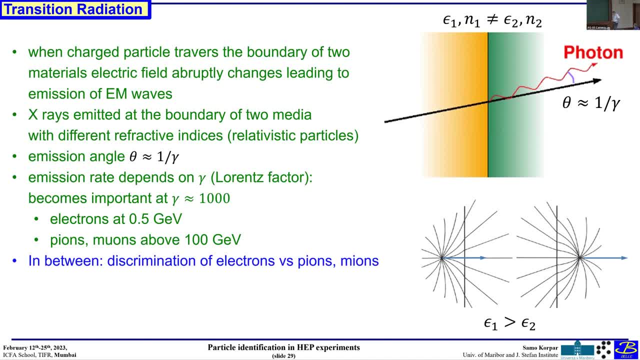 happens at the boundary of 2d electric media with different refractive index or different speed of light. so when charged particle goes over such a boundary, you can actually statically plot the field electric field at the boundary by using this charge mirroring technique. so you had to add: 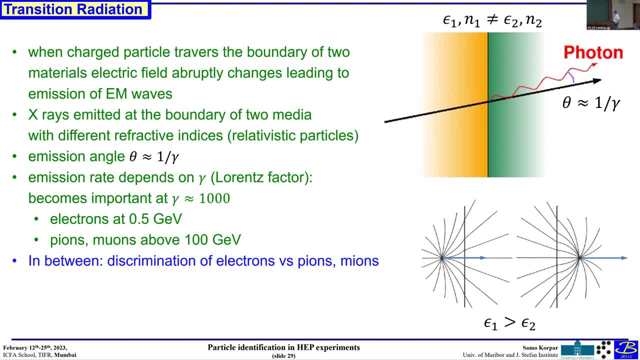 additional two charges to make a combined electric field. on the other side the field is based on the basically the same shape as for the one charge and on the side where the charge actually is, its combination of two charges from one and the other side. so there is a 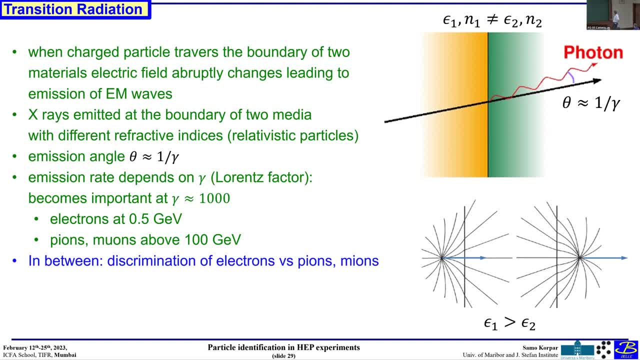 change in shape when the particle goes from this side from the others, these two charges change and the shape of the field also changes in one on the other side. so there is an abrupt change of electric field which in principle is change of the dipole also. uh, of this. 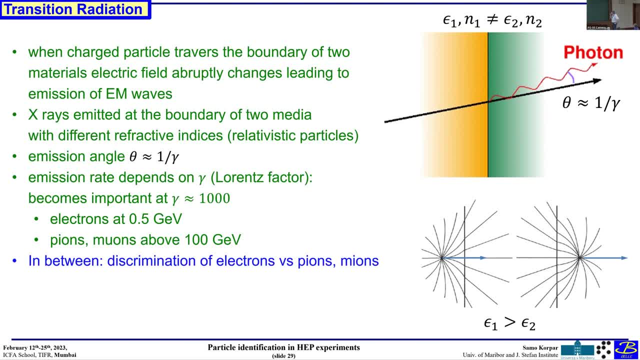 imaging charges and whenever this happens we have emission of electromagnetic waves. now the formulas are pretty complex, but the main thing is that at the high momenta, where we have get enough of these photons to be useful, uh, the angle is very small actually. we are talking about a. 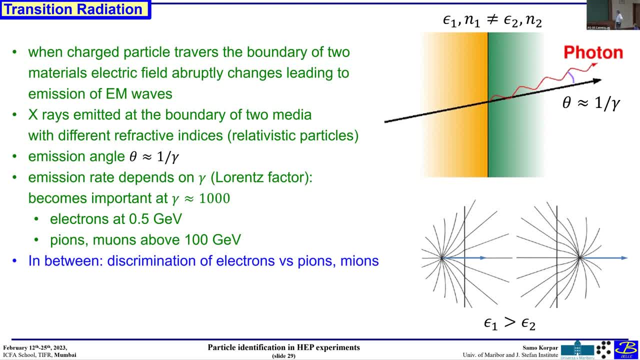 lawrence factor of 1000, so it means that this is, uh, on the order of milli radians. so it's basically the photons that are produced by the electrons that we use. actually, more or less on the short path, follow the particle trajectory and also the emission rate. 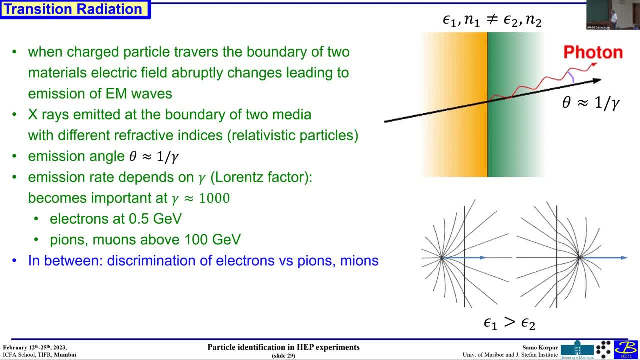 in the single boundary also depends on the lawrence factor, so it becomes basically significant to the point that you can actually detect it at gamma factors of around 1000, which is only more or less reached by the electrons. so it's then possible to eliminate electrons from. 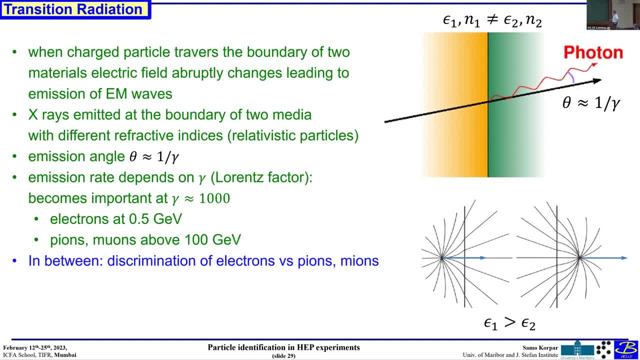 let's say pions or muons or some other heavier particles. so electrons reach this at half a gv and pions and muons at about 100 gv. in between these two, basically, you get some separation or rejection of pions and muons against the electron. 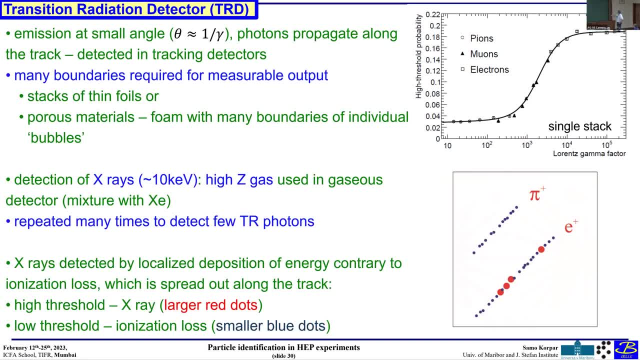 hypothesis. so emission angle is small and the photons actually follow the correct trajectory. many boundaries are very important to get the measurable output because the single boundary, the probability to get the photon and these photons are at that momenta in the x-ray range. x-ray range: uh, you have, you need. 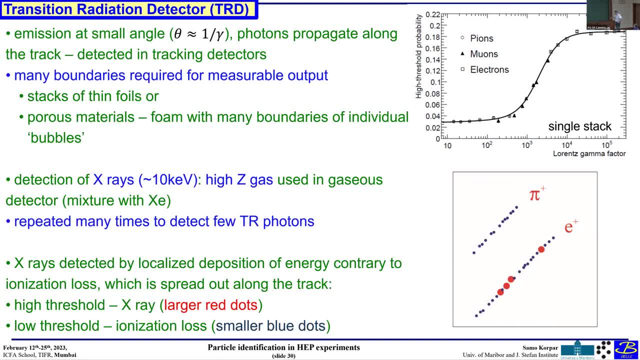 to combine many photo boundaries on the order of few tens, but then at some point the saturation happens, so it doesn't make sense to make a very long sandwich of these- uh, different materials. so stacks of thin foils are used all the time, or even the porous material like fibers. 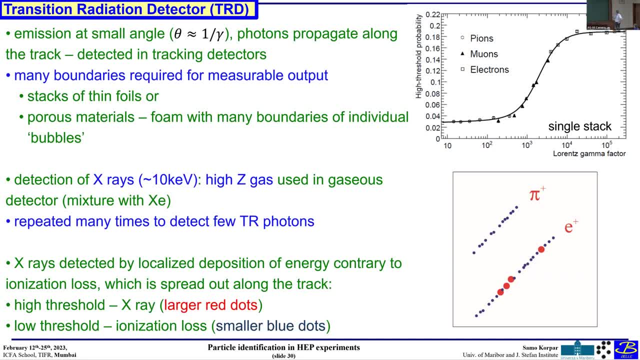 with the air in between, or some kind of foams with the bubbles in, can be used to actually make the material where this radiation is produced. and a single combination of one stack of these foils or thickness of this porous material and the detector behind you can see the probability that you 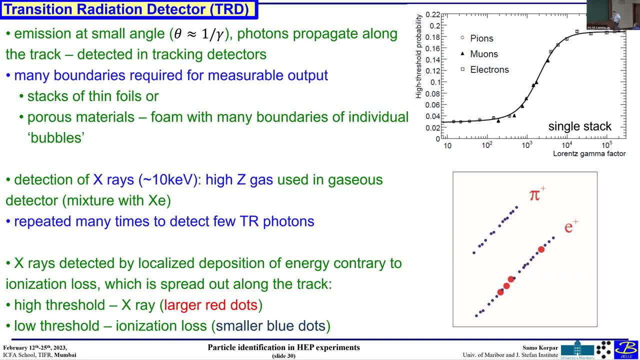 will actually detect the signal with in the gaseous detector that is behind the signal of this x-ray produced. and this actually starts, as we said, around gamma 1000 and then goes up and then reaches some saturation, and this is around point two. so it's. 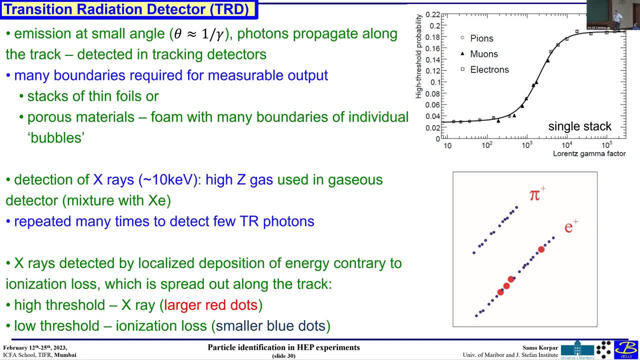 not very probable that one such stack will produce one photon, so you need also then combine many layers of this to make a detector that will then detect uh more, and this is done by gaseous detector with the gas mixture that uses uh gas with a high z. 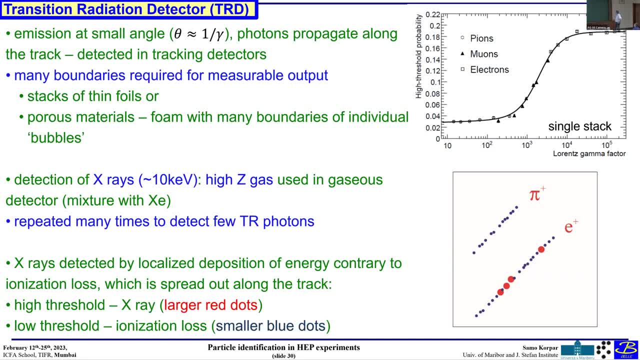 like xenon, let's say xenon, co2 or something like that. and in xenon then this tank ev electrons are converted to photons, are converted to electrons. kick out electrons and then these electrons for it, because they are low energetic, they will make a bunch of ionization very close to 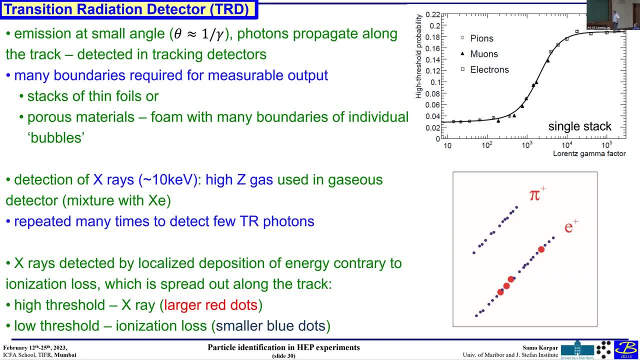 together and this will make then the large signal when it reaches the anode wire. so looking at, let's say, the track we will see later, the track of the pion that goes through such a detector, you will get a small ionization. maybe from time to time you get high. 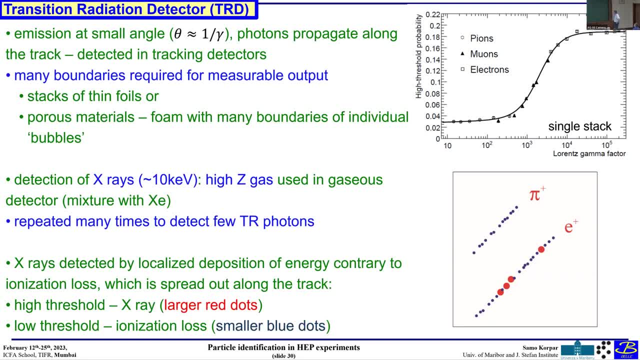 energetic delta electron, which will fake this x-ray, but otherwise you get low signals and then, when the electron goes through such a detector, from time to time you get the radiation, radiation photon, and then you get the large signal and this then separates basically these two. so this: 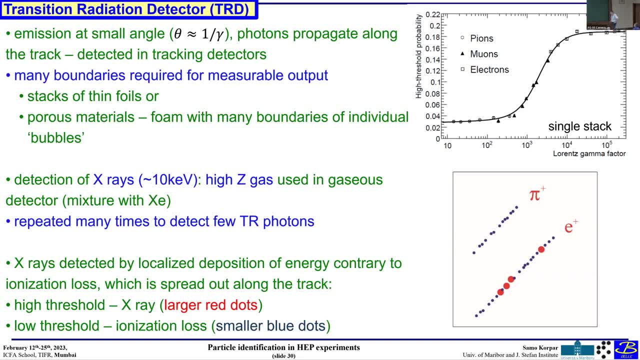 and this is done basically by then using the two different thresholds to detect or to separate the low and high signals. so it's usually called then the high threshold and low threshold signal on the graphs. that's why it's written here an example. there are two examples. 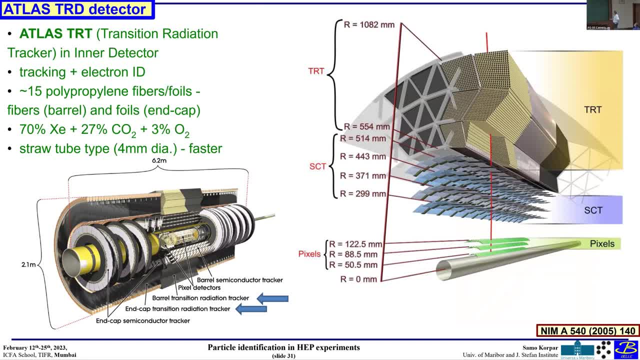 used in lhc, so atlas transition radiation detector is actually the tracker at the same time. so these are not usually a dedicated uh pid devices, but used also for tracking because of course they also measure the tracks. so there are 15 polypropylene fiber foils. 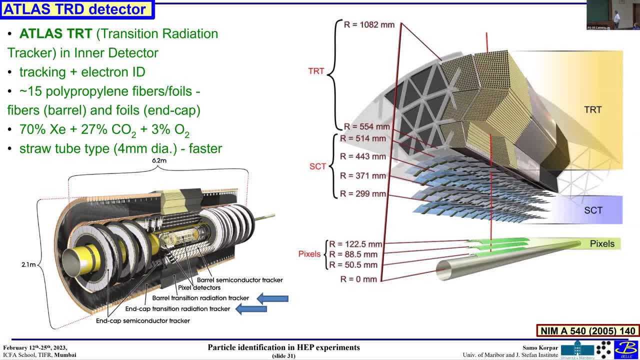 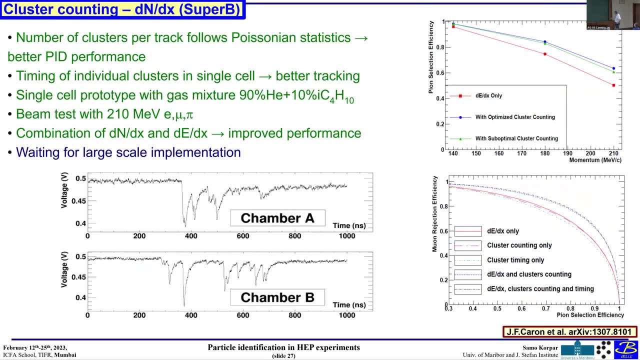 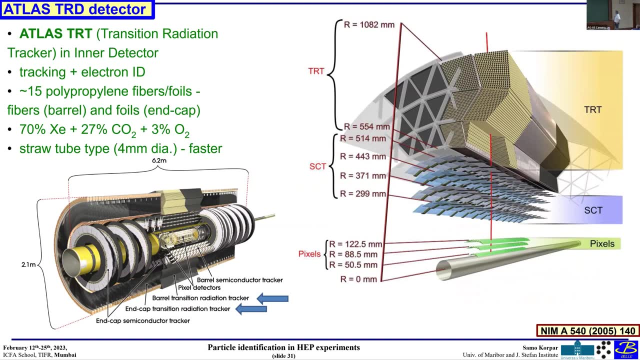 in one cell and then, oops, the wrong button. okay, so this is a different uh top. there are foils and then there are uh fibers, uh, at a different position, barrel and that cup barrel around here and then cup somewhere here. so these are two with blue arrows, these are two detectors. 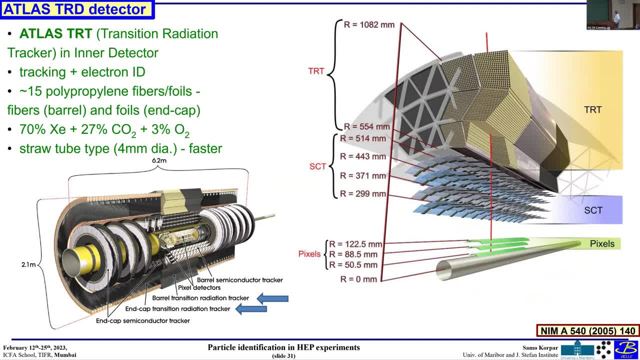 basically in inner part of the atlas experiment. so the straw tube four millimeter diameter is used to get the fast signals out and this is the gas mixture that is used in the detector with xenon to convert x-rays. so this is the position basically. this is only this inner part and you can see. 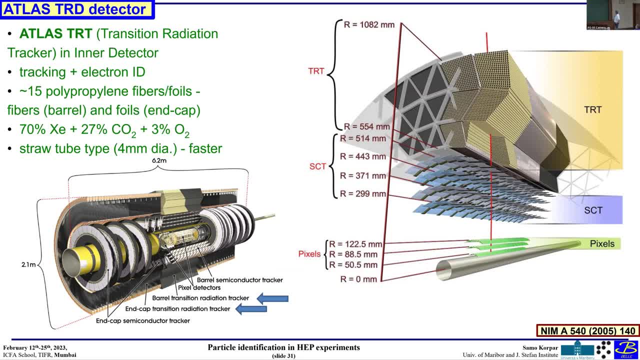 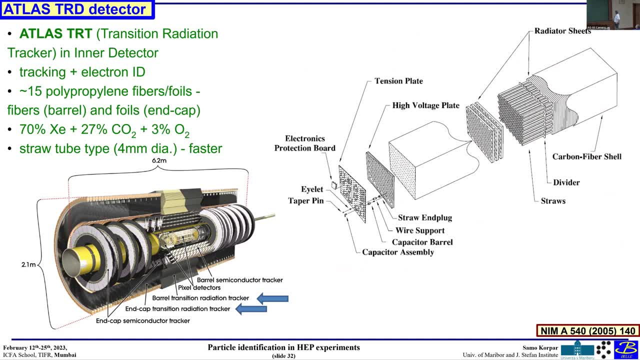 the tracking detector and the final tracking is basically a combined combination of transition radiation and tracking the detector. this is the cell, so there is. there are these foils or fibers inserted over the stroke straw tubes and in this, when track travels through, produces x-rays and this then makes the 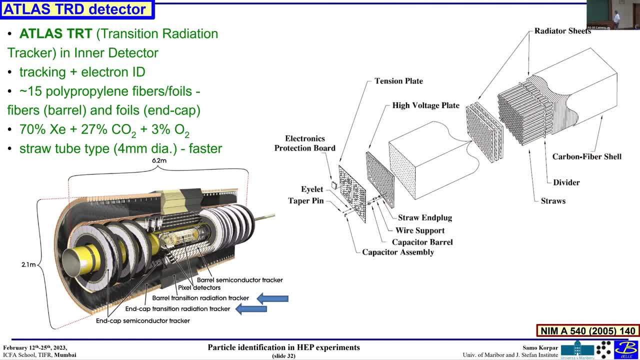 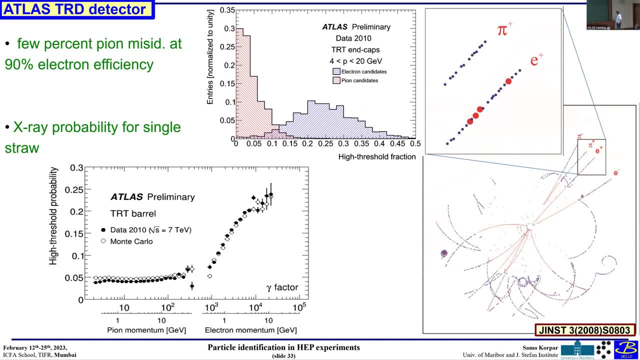 extra signal in the straw tubes that uh are inserted in part of the detector and uh, this was the picture actually from here. this is an event with the inner tracking and then this uh outer tracking somewhere here, and then this is actually a part that is shown here. so when the electron goes through, 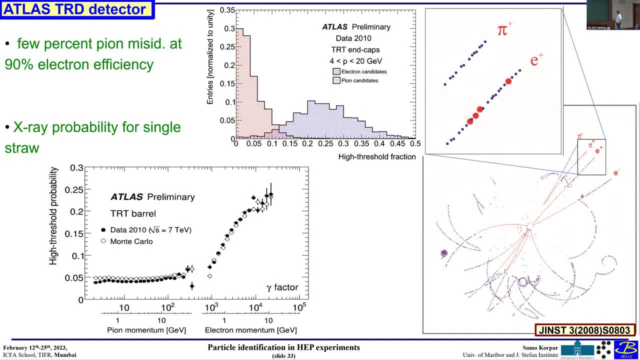 you get these extra signals. where the pion goes through you don't get, there is another electron. so you can see the red dots on this. so it identifies the electrons and this is basically how the distribution of the pulse height actually looks like and you can see that there are. 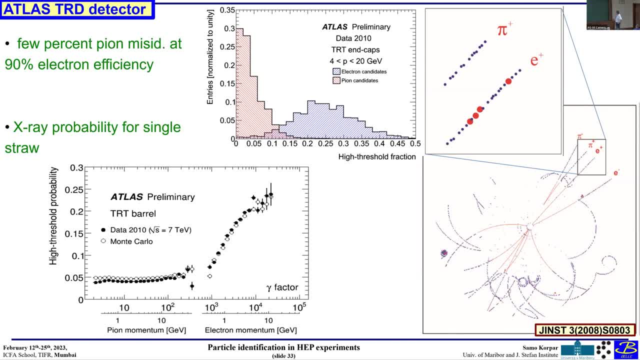 low signals for the pions and you get the higher signals from the electrons. of course there is always some overlay, overlap of pdf distributions, probability, density functions, and this means that you get some, let's say, 90 percent electron efficiency, a few percent pion misidentification and 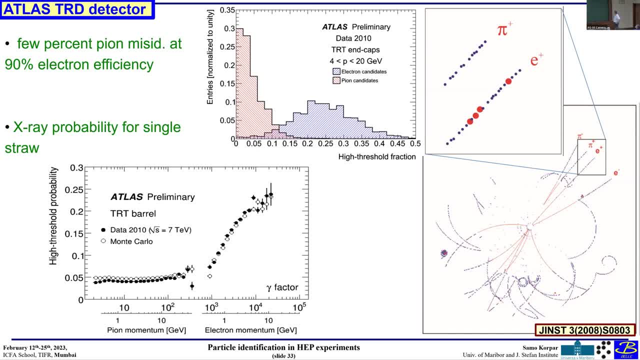 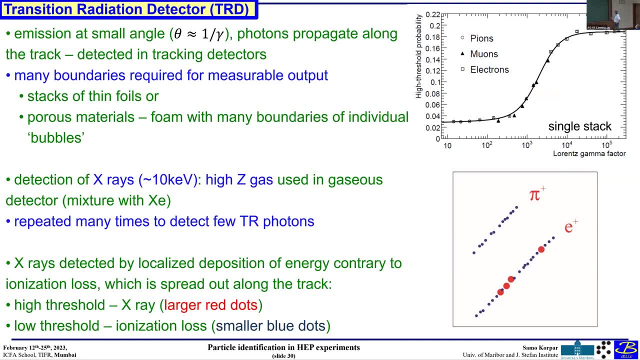 multiplication probability. and for these straw tubes this is a similar plot as i showed before. before actually it was uh for some more general test detector. and you can see for different parts, actually different pions, mu and electrons all behave basically at the same way when they reach the same lawrence factor. 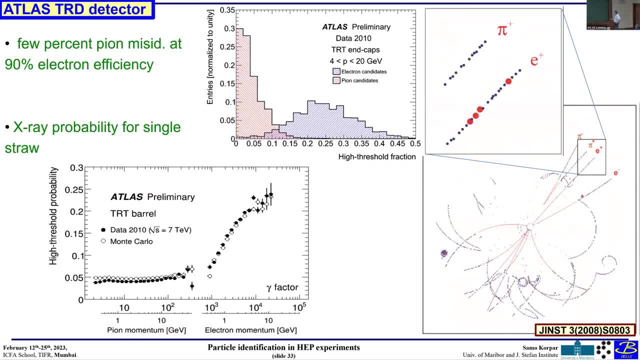 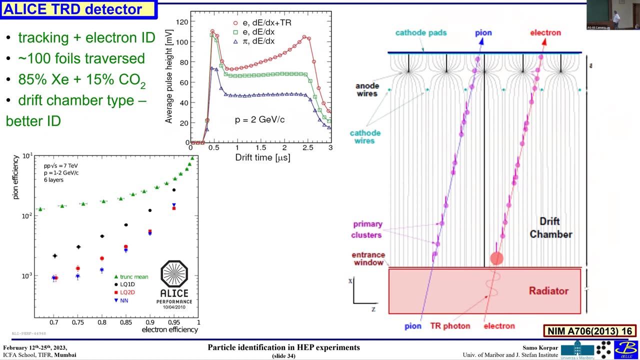 and here is just for the atlas experiments, you can see the similar distribution. so for electrons you start to detect large signals, which gives you the separation, and in alice there is a drift chamber. basically so there is a longer drift path and in each cell of such a drift chamber there is a 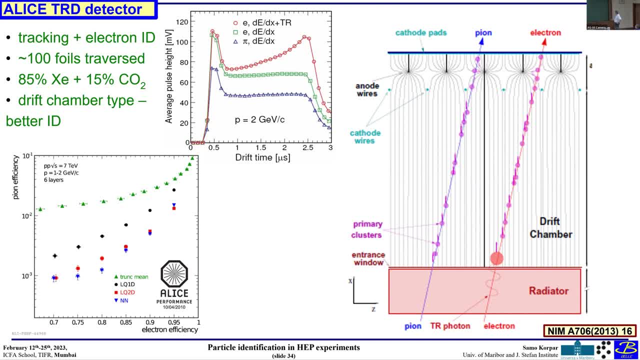 foil in front, a hundred foils basically sandwich here and then when the pion goes through, there is no transition radiation. when electron goes through, you get the x-ray which is quickly absorbed, basically in the drift chamber and drifts a long time. so you can then 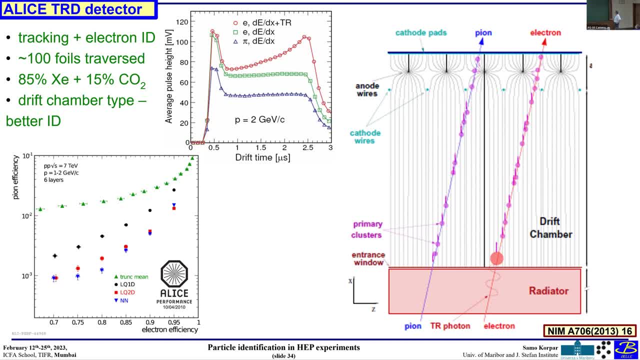 separate the signals with the transition radiation signal because there is a large signal at the end due to this x-ray deposited at the very beginning, but of course not all are immediately here, so you have kind of exponential decay. but this is the average signal with the transition radiation electron. 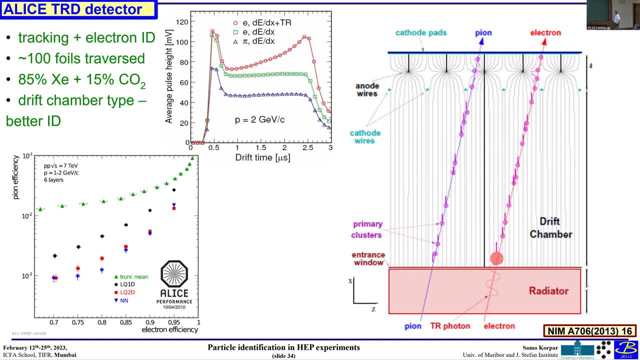 and there are different techniques. truncated mean some kind of likelihood, neural networks that then give the separation. so if we look at the 90 percent electron efficiency, we are at the percent level, or even below, of the misidentification of pions in this detector. so it works. 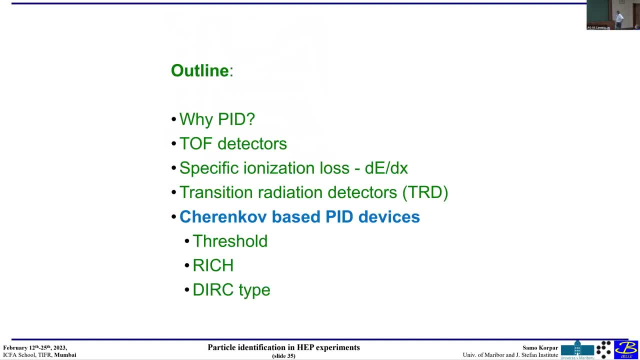 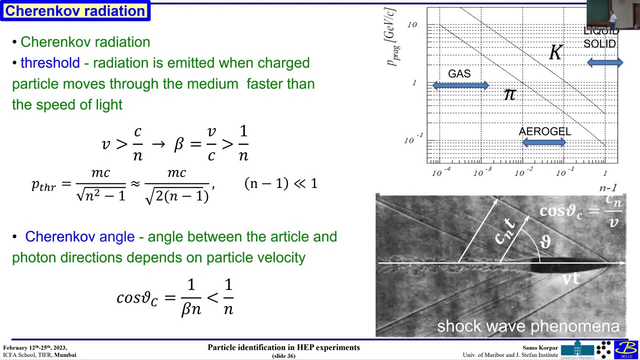 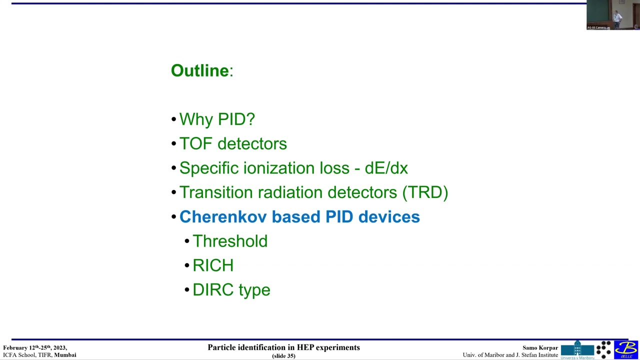 very well, okay. so, yeah, yeah, okay, i'm basically looking at the. yeah, okay, i'm basically came through the program of the first day, uh, so, uh, tomorrow. now we can say a few words already today about the general properties of the alec of the cherenko light. 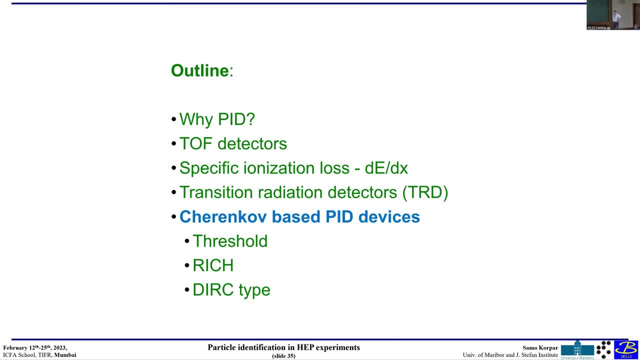 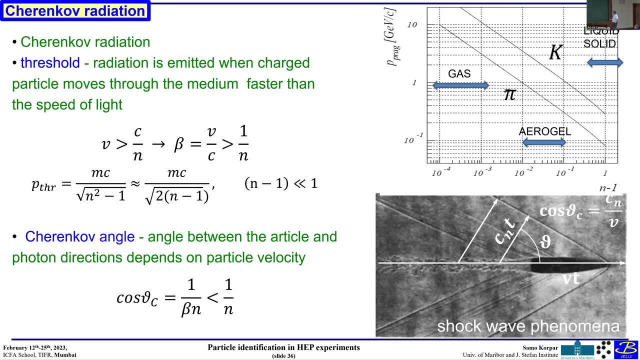 and then tomorrow we will have the detectors to to use this five minutes, yeah, uh, so the chernico. there is unfortunately something missing here. the chernico detector is produced when the charged particle travels through the medium, through the dielectric, with the speed that is higher than the. 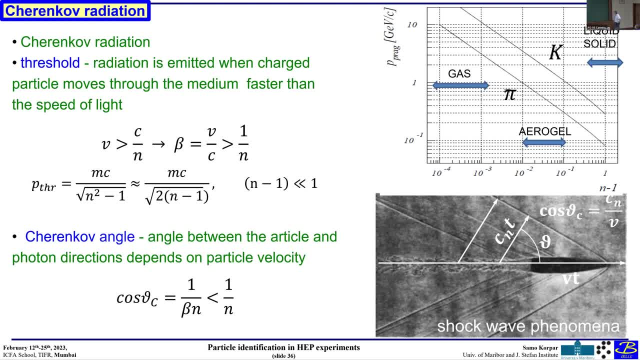 speed of light in that medium, of course, which is lower than the speed of lighting light in vacuum, which is the limit. so, uh, this is basically a shock wave phenomenon that we are familiar with from the mechanical waves, like sound waves in the air or waves on the water, or so. 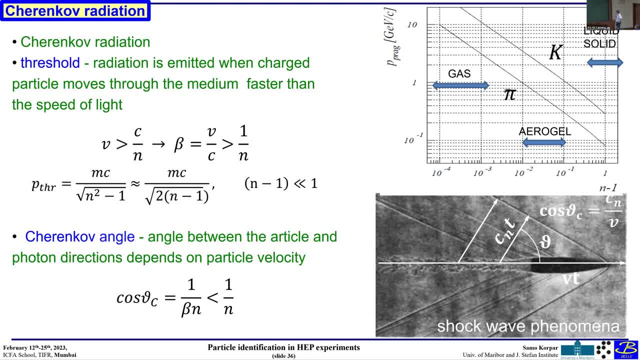 on. so this is a picture basically of the bullet traveling through the air and you can see the shock wave formed due to the change of the refractive index in this front. you can see the boundaries where the actually the wave front is traveling of this bullet. so 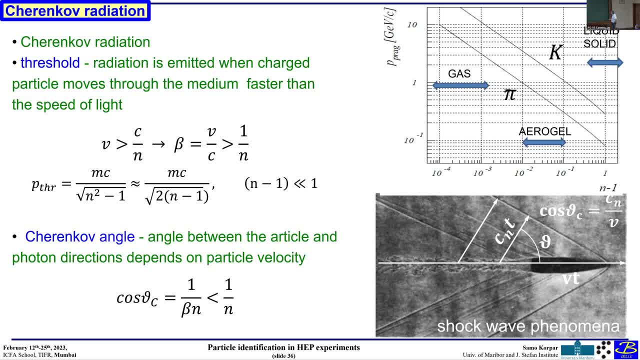 as we are used to for this shock wave front, we can basically calculate the angle at which it happens, because the waves from the, from the track travel, propagate with a speed of- in this case sound, but this is the speed of light in the medium CN, and then the particle travels faster. 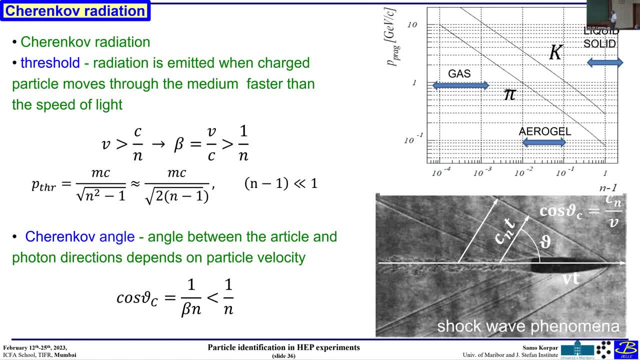 with this speed and we get this rectangular triangle, and the cosine is then the ratio of these two speeds. So this gives us the angle at which the wave propagates In the Cherenkov light. this gives you the angle at which photons are emitted from the track. 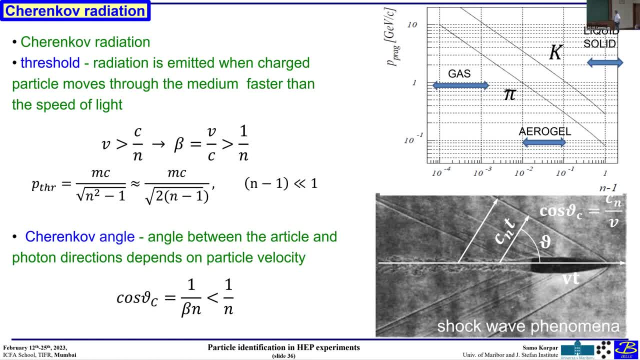 And this is the angle that we measure them, to then come back to the velocity of the particle. So there are two effects. One is obvious, it's basically the threshold. The threshold is because the velocity has to be higher than the speed of light in the medium C divided by N. 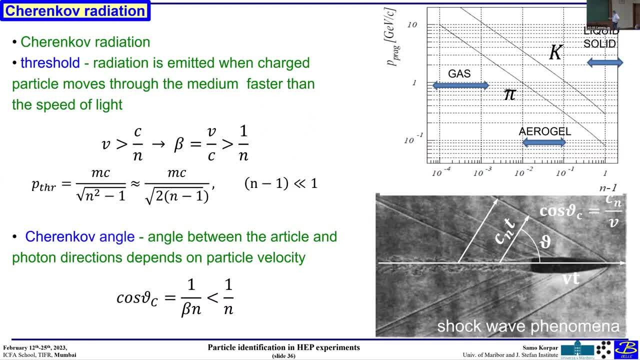 Oops, And it means that then the beta is, which is V over C, must be larger than one over N. So this is the limit which gives you then the threshold momentum, and the threshold momentum, if you combine these formulas together, is the momentum M- C. 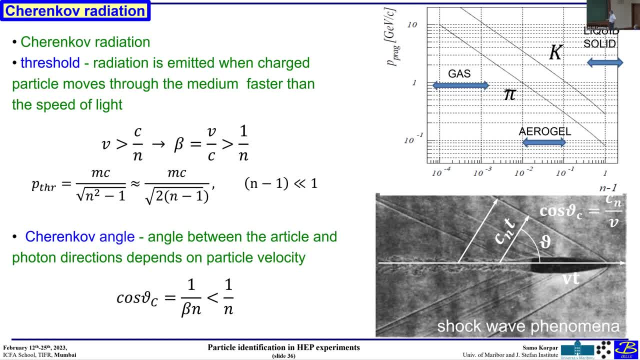 basically the mass times, the speed of light divided by square minus the speed of light divided by square minus the speed of light divided by square minus one. So this is the formula for threshold, And when the momentum is high, or trash, or reflective index, let's put it this way: 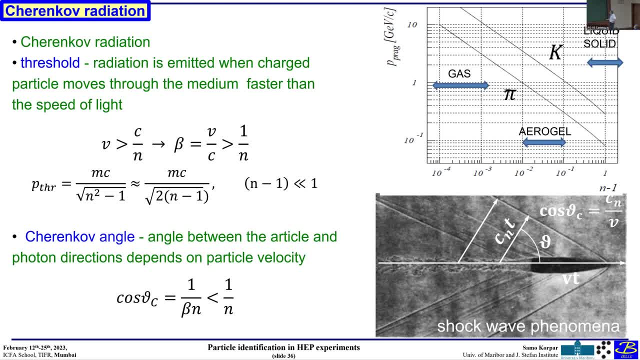 Reflective index is small, Then for gas, let's say: then we can actually make approximation in this way. So the plot on this side is this: threshold- Sorry, this is Slovenian practice- threshold momentum And as a function of N minus one, 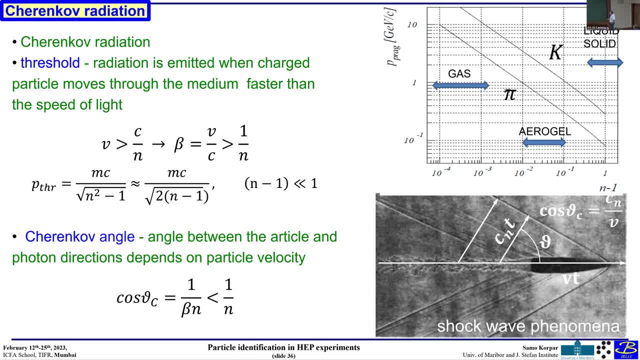 So zero would mean actually more or less smaller. This is comes to the air or the gases, And the larger it is to one means actually two. these are some heavier crystals like PBF, two or so. Of course diamond has much higher, and so on. 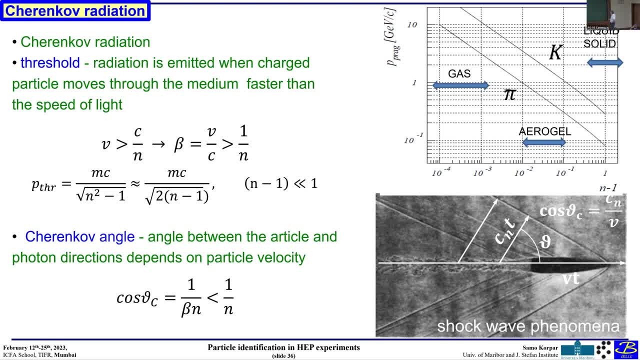 So they are higher reflecting in the indices, but usually not used. The glass is somewhere here. yeah, 1.5 or so. So this lower part is covered. Reflective indices is covered by gaseous detectors. One could extend it by high pressure. 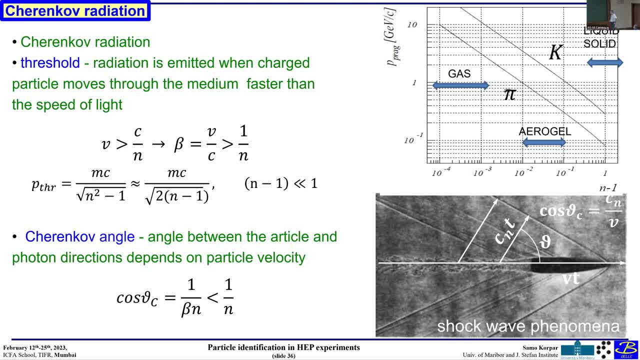 but this is actually much more work for large volumes, So it's not usually done. Then there is a solid and liquids which have roughly the same refractive indices. I think the lowest one is a sodium fluoride, which has roughly the same refractive indices. I think the lowest one is a sodium fluoride. 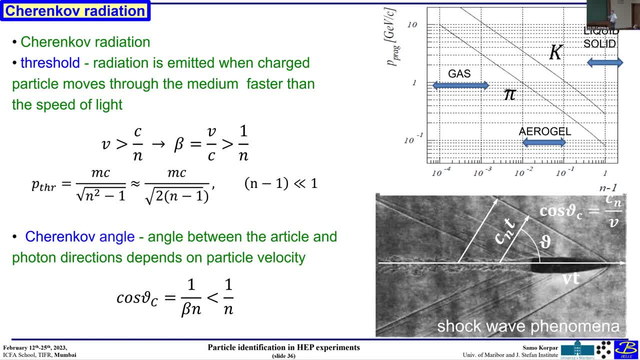 I think the lowest one is a sodium fluoride, solid 1.27 or something like that, And then upwards. So this is covered by liquid or solids. And then there is aerogel, which is a kind of material made out of silicium oxide. 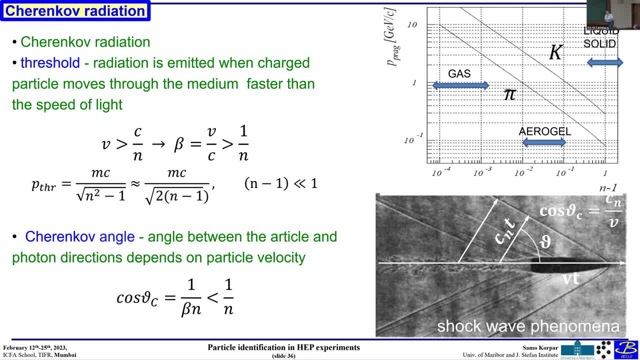 So it's basically a glass with a lot of air inside. At the lab that we have, you have seen the two samples of aerogel tiles that are used as a radiator. So this is basically the materials that are available for different ranges. 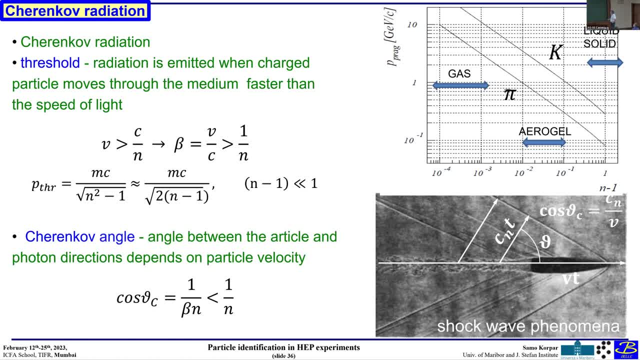 And this threshold effect can be used to discriminate on binary basis. So whether the particle radiates, then it's lighter, If it doesn't radiate, then it's heavier at a certain moment. So this is the threshold. Cherenko detector. 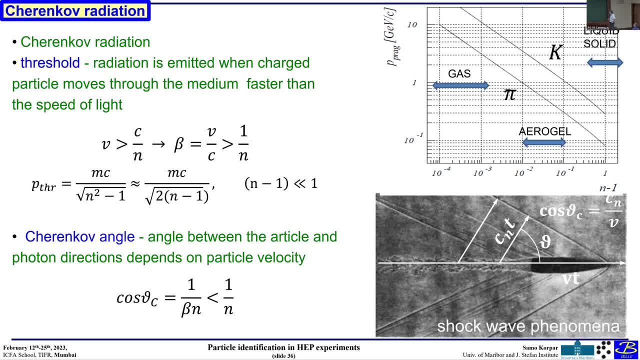 And then the other thing is Cherenko angle, So each photon actually travels at a certain direction with respect to the, the track, And we can measure, basically if we know where the photon roughly was emitted, and then we measure the point somewhere else. 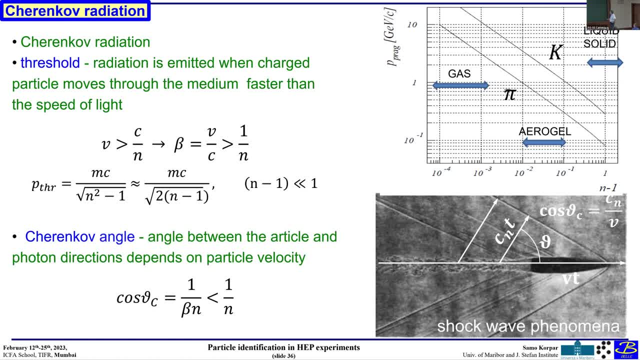 we can reconstruct the photon path, And knowing the track of the particle, we can then measure the Cherenko angle And this gives us a better estimate of velocity. basically, Then we can separate. also, when both particles start to radiate, we can still separate them for some time. 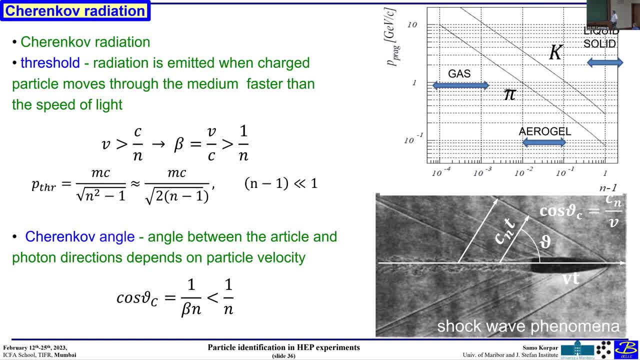 because we can measure the difference in the Cherenko angle. So, yeah, Okay, let me finish just with this introduction of Cherenko light. So tomorrow we will continue with Cherenko light properties and then several different kinds of detectors. 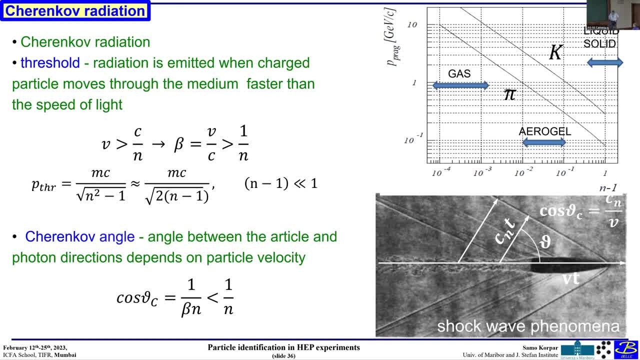 that use, basically Cherenko light, Thank you. Okay, Thanks, Samuel, For a nice introduction to particle ID and some of the detectors. Yeah, Now floor is open to for question. Why do you need a dedicated electron ID? Because can't you just identify it using the track? 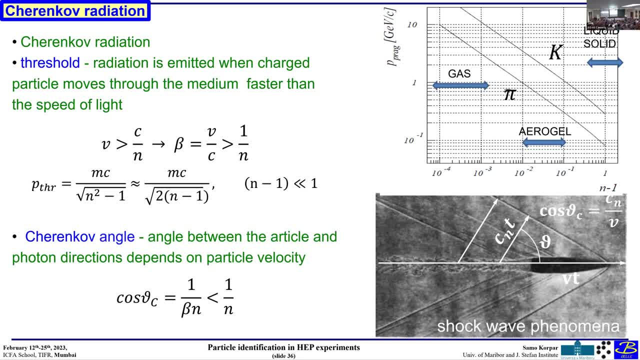 and the signal in the ECAL At very high momenta. I guess there is not much difference. I mean, it's not a lot. of other particles also reach the same ratio, basically beta one. So at high momentum you need some other. 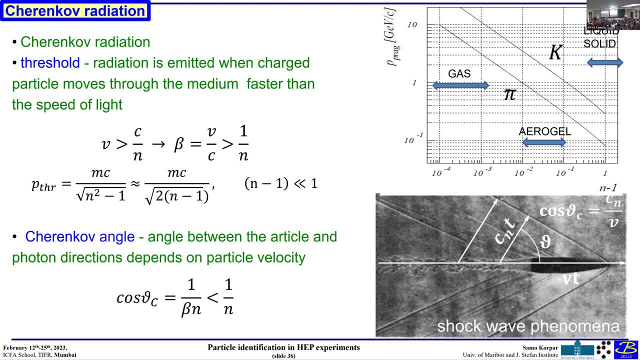 and also they don't stop anymore in the color. Okay, We're saying so. you need some other technique at work, but this is at very high momenta. Okay, Very nice talk. I want to ask one question that: is there any possibility? 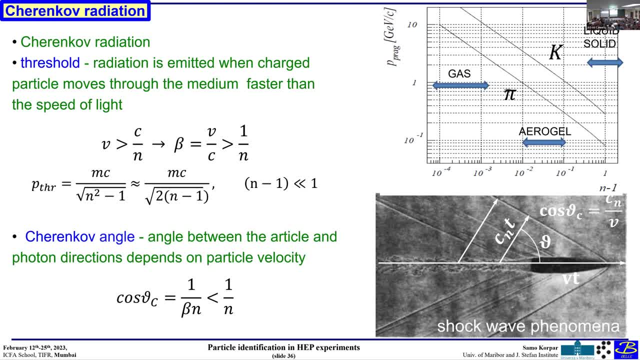 to detect the weekly interacting particles. Okay, Is there any possibility to detect the weekly interacting particles like exons or other particles, not really that you mean like neutrinos or yeah, yeah, basically, as you know, this is basically very, very rarely interacts. so of course there are special detectors for neutrino physics that. 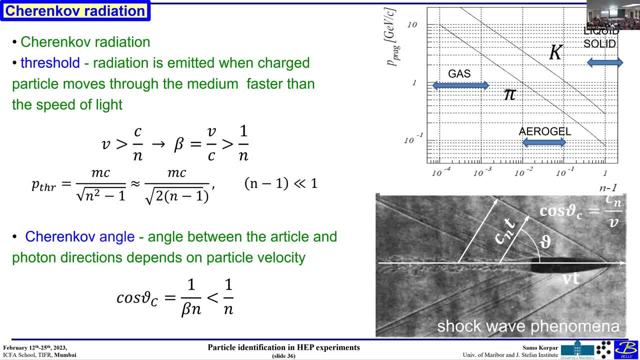 use a very large volumes and then after interaction you actually reconstruct this by detecting electron or whatever is produced, muon in this interaction with the matter, but directly with weak interaction you don't. I mean. detectors basically detect either hadronic interaction with nuclear or electron, electromagnetic interaction. on what does the amount of Cherenkov light? 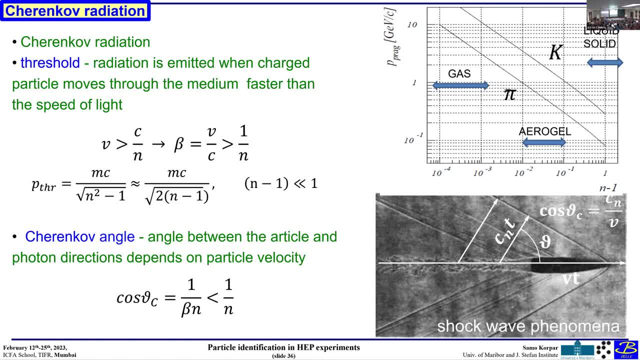 produced depends on. I mean, what are the factors on which this depends on? this is actually the next slide, so, if you allow me, I will postpone this for tomorrow. okay, thank you? thank you, professor, for your wonderful presentation. why the muons particles moves faster than Cherenkov light? it is only due to low range. 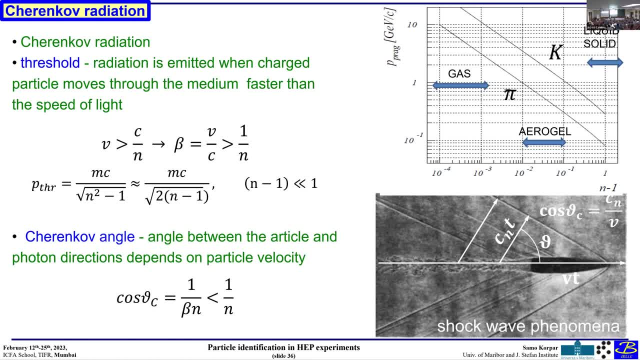 factor or something else. when the neutrino interacts with the atomic nucleus of the medium, it can produce charged leptons such as an electron, muon or tau. but why? muon neutrino is of high research interest than others? initially, in spite of its heavier mass. it was, yeah, we'll talk about later. yeah, I didn't sorry, I didn't completely understand. it was long. 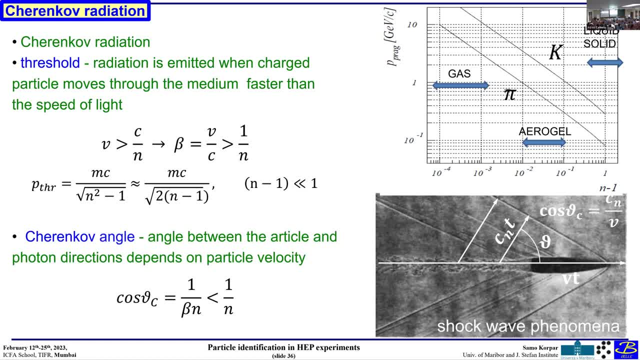 question. I had parts of them I didn't understand. it was about: okay, I'll make sort of that- why we can discuss maybe later so that you can explain me what was exactly the question. so, like particle identification, can we do charge identification without external magnetic field, just simply using the energy loss mechanism? charge identification, yeah, I mean positive or negative. 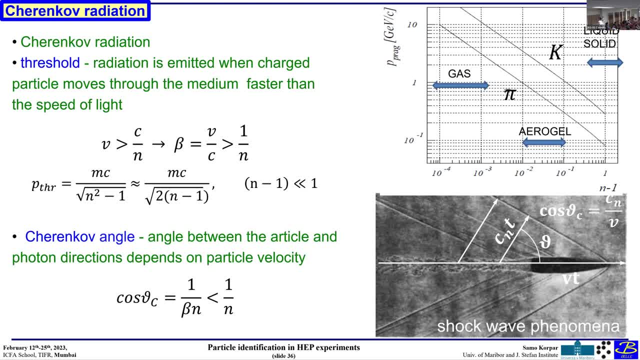 yeah, let's say muon or antimuon. so in principle they will interact differently in a matter because of they have different charges. so can I use that future along with their? in that momentum probably very small difference would happen. I mean, when they stop in the medium, there is some difference between one and the other. 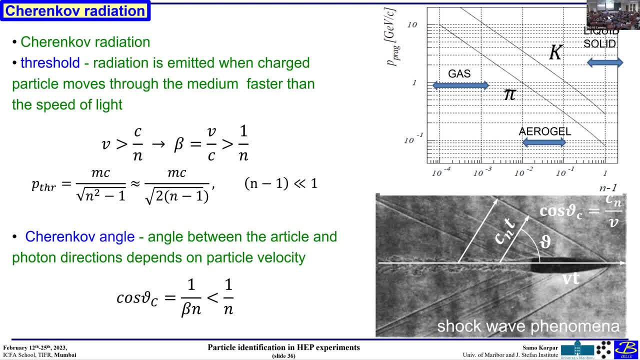 particle, but when they travel fast through. I don't think one can use the response of the detector to separate particles from antiparticle, I mean from strongly interactive particles. there is some asymmetry in the interaction but it's hard to say. I mean you can, on the average, say that there is a difference for 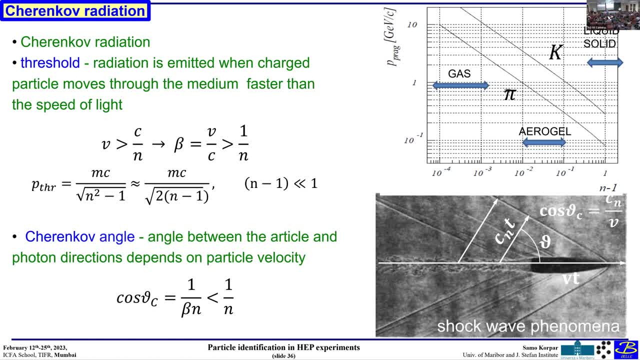 kaon or antikaon when they travel through the matter, because there is more matter than there is no antimatter in the material. but on the event by event basis, I don't think there is a very much difference. is that, uh difficulty comes because of the limitation of the detector or is actually from the interaction? 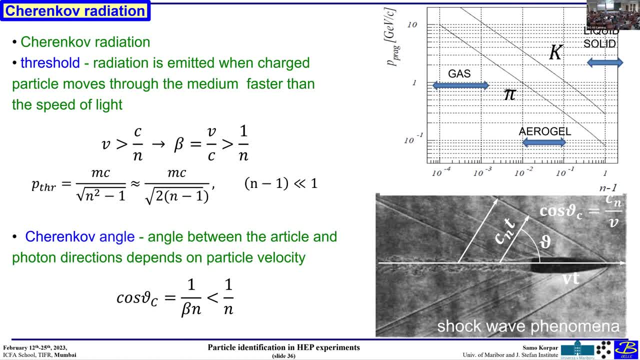 mechanism itself is very small. which one so is that limitation comes because of the director performance. so as he says that only for this k on, let's say k plus and K minus the interaction of the materials. there is a slight difference, but there is a very small difference, that in this detector